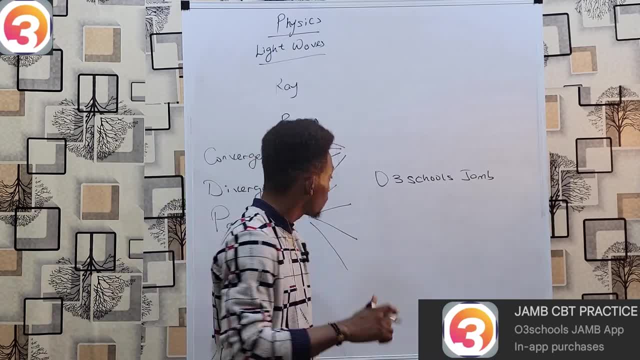 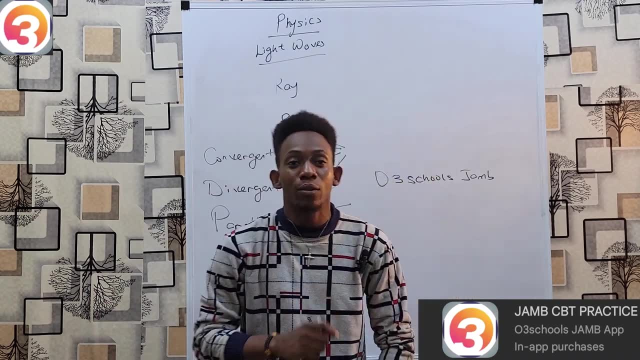 Parallel beams, however, can be gotten with some of our torch lights, and those are the types of beams. Now we move on From knowing this. the most important thing we must know about light is that light always travels in a straight line. Light does not curve around objects, except slightly in. 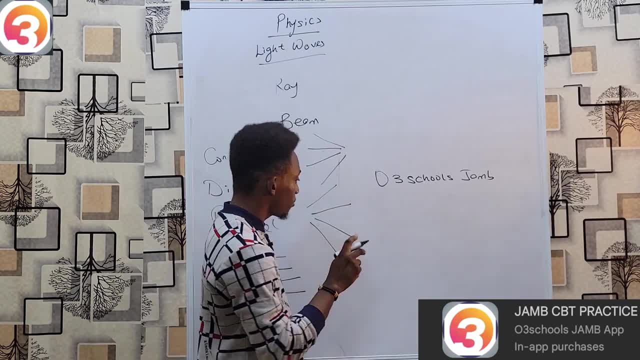 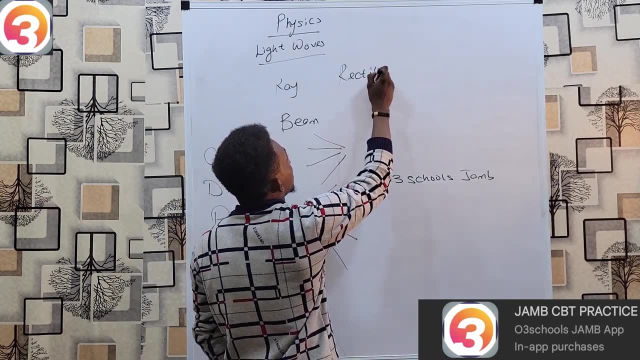 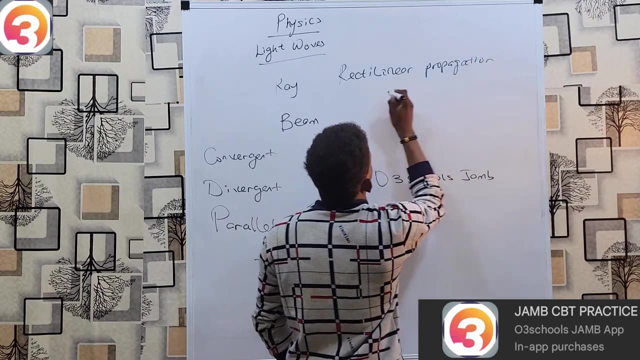 diffraction, which we have looked at in the previous topic. So, like I was saying, light travels in a straight line and this phenomenon is referred to as the Rectilinear Propagation of Light. Rectilinear Propagation of Light: The name might sound big, but all it says, quite simply, is that 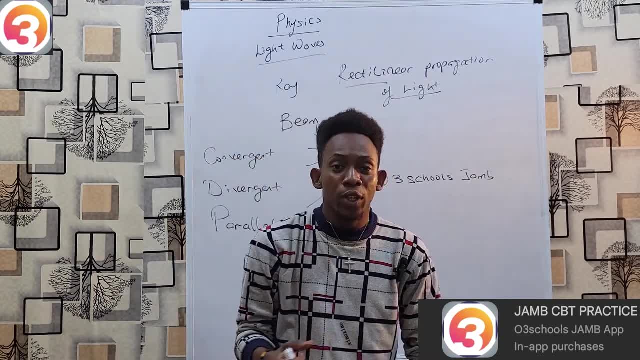 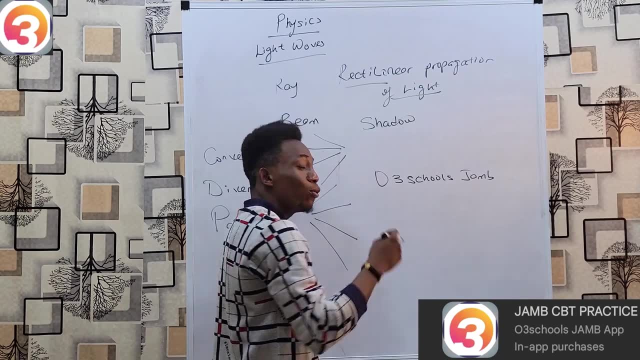 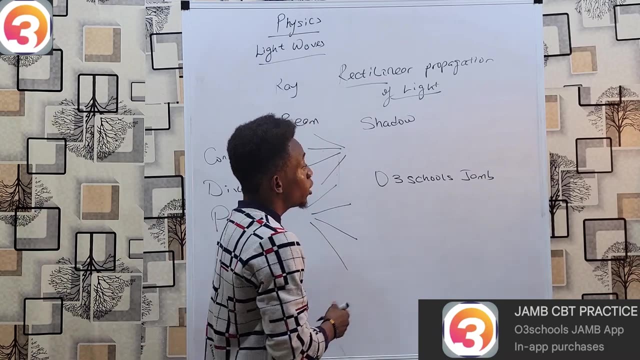 light will always move in a straight line. Now, there are several effects of this movement in a straight line, and the most obvious one is the shadow. We've all seen our shadow at different times. At times the shadow appears long, At times it appears short. What creates the shadow? The shadow is. 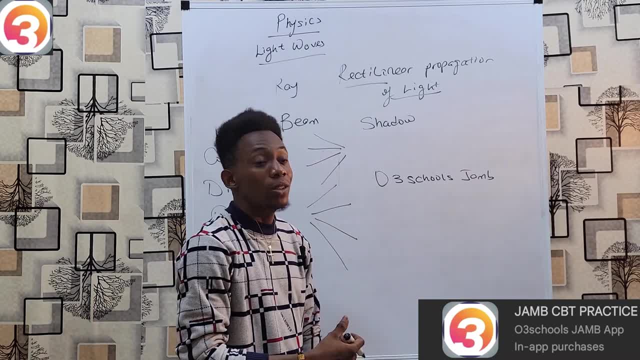 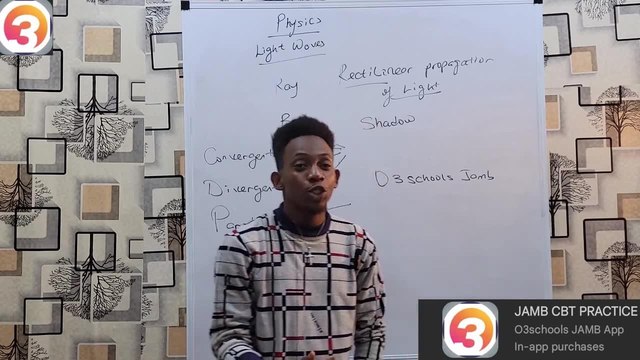 created because the human or the object within the shadow is opaque. It prevents light from actually passing through him and reaching the space behind, And for that reason you have a dark space in the shape of the outline of the person, and that's what we call a shadow. 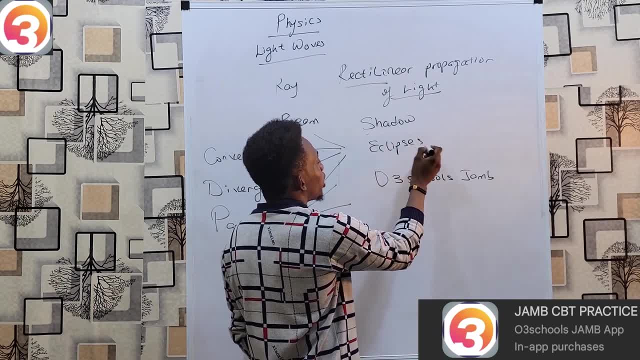 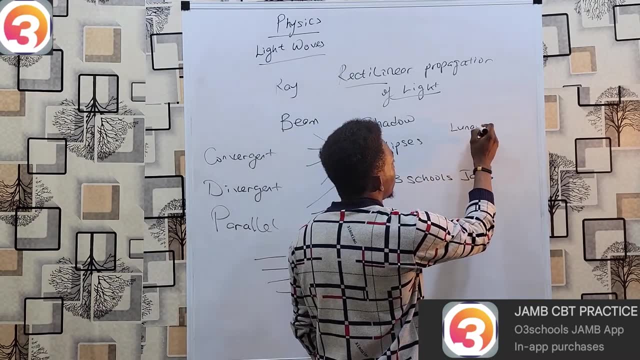 Now we also have eclipses. Eclipses are like shadows, but eclipses are shadows caused by celestial objects. There are two eclipses we can experience here on Earth: The lunar eclipse and the solar eclipse. The lunar eclipse is the eclipse of the moon. and that occurs when the Earth goes between the sun and the moon. and the solar eclipse, or eclipses of the sun, is one To see architecture, in other words, to see how something like a globe, whether it is its position in the earthartaufen or in itsts center, shots. 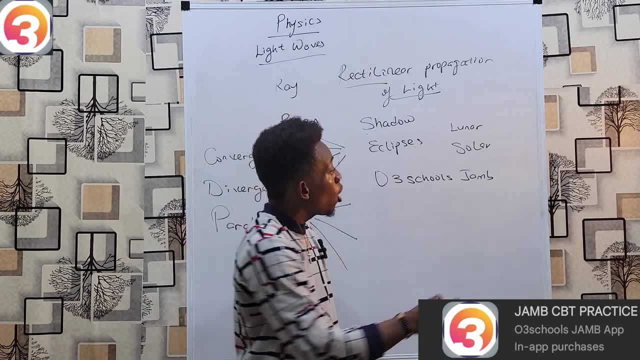 The solar eclipse exists because when it goes between the sun, the eclipses occur between the moon and the earth and the sun and the eclipses occur when the posts enter the moon. moon and solar eclipse or axis of the sun occurs when the moon gets between the earth and 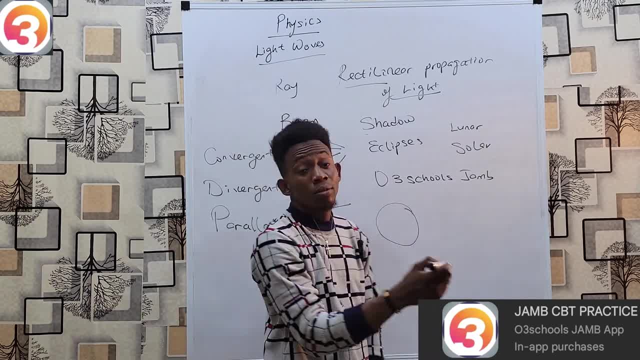 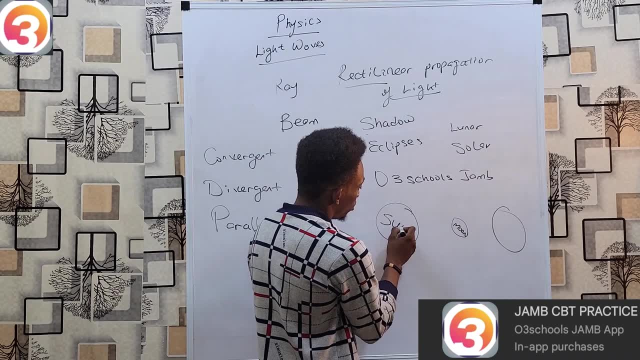 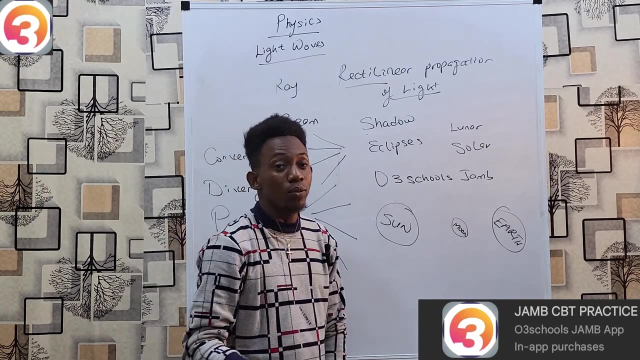 the sun. in that case, you may experience a few minutes of darkness during the day. this is the moon, this is the sun and this is the earth. now, once you're away, the moon is a non-luminous body. the moon doesn't give up any light. 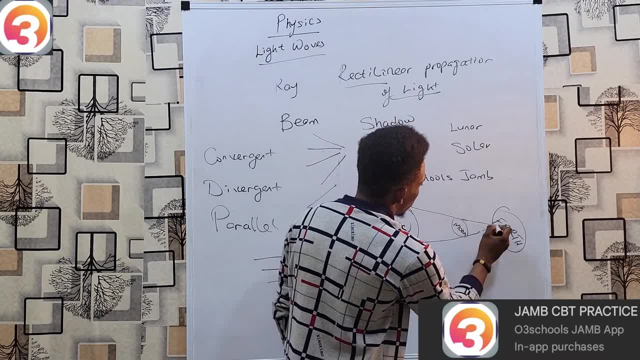 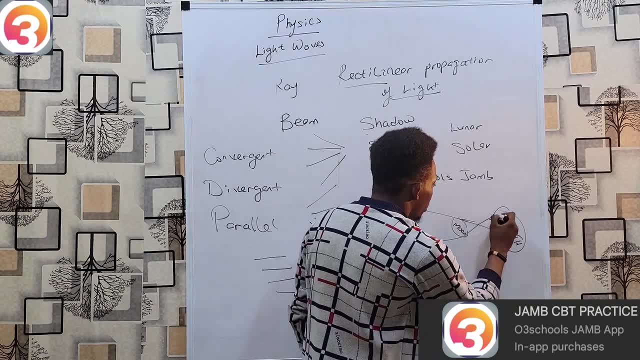 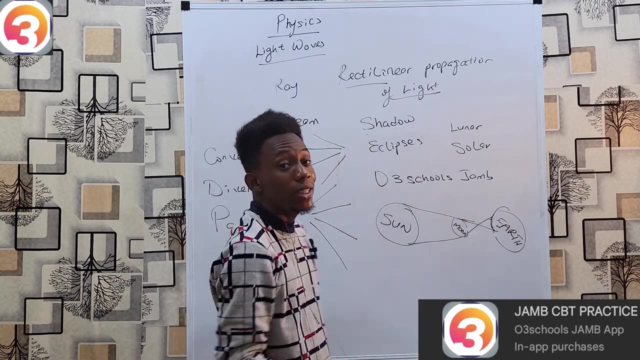 and for that reason, if it is to step between the sun and the earth, light is unable to reach certain parts of the earth, and those places experience darkness. and that tells us that we have two types of bodies existed. naturally, they are luminous bodies and non-luminous. 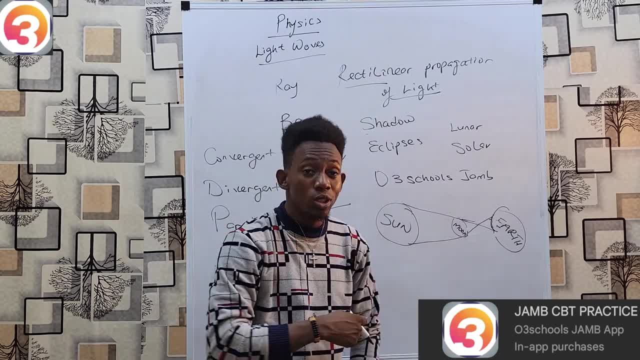 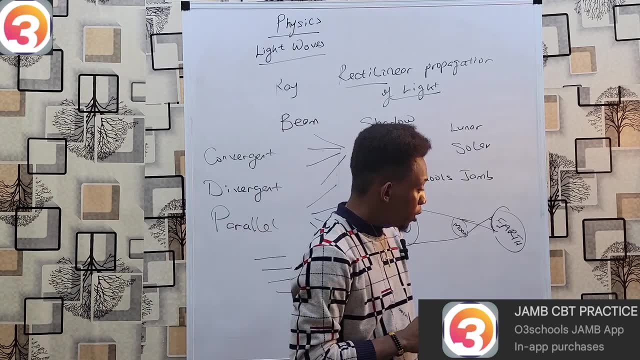 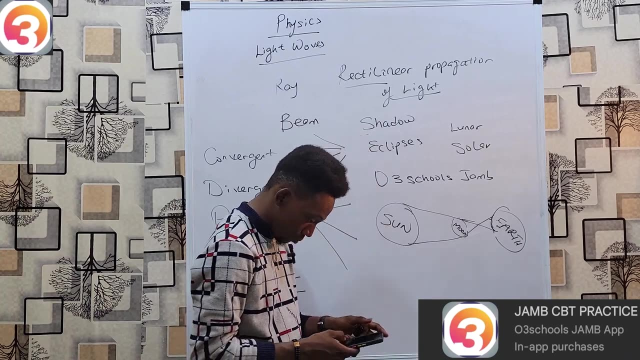 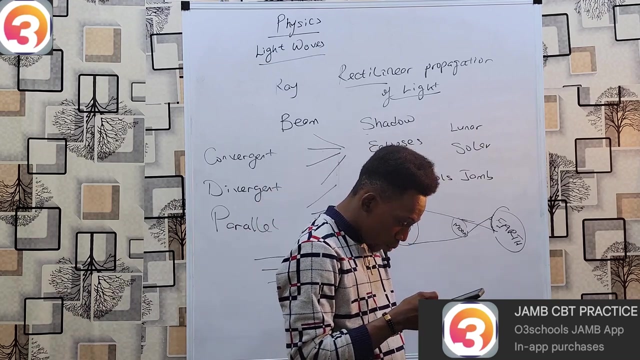 luminous bodies are those that can produce light of their own, eg the sun, while non-luminous bodies do not produce light eg the moon. okay, and from this point we can actually take a question from the app. now the question is quite simple. on searching your app, you can find this. 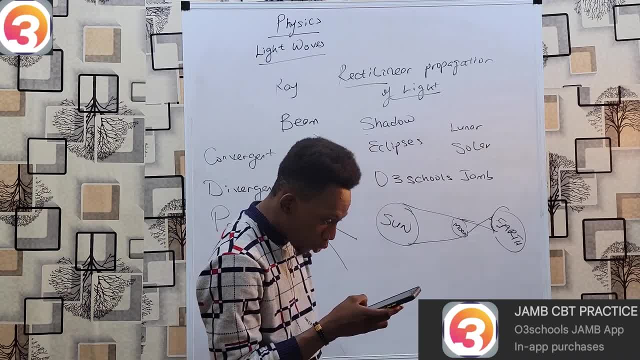 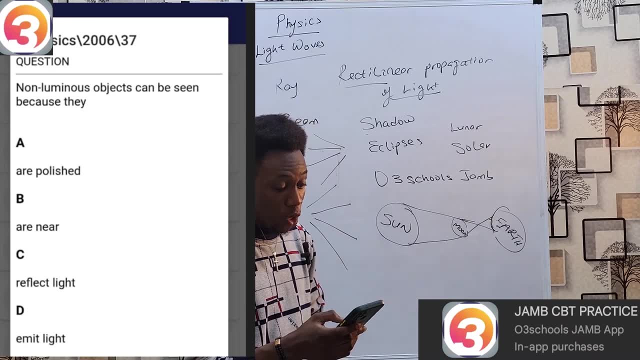 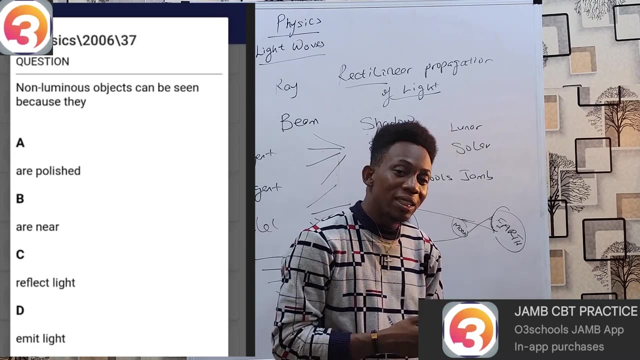 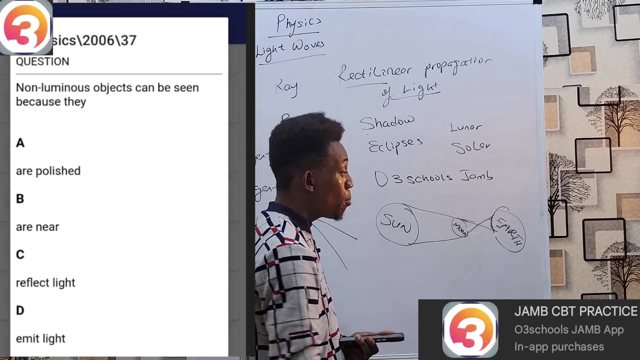 question in the year 2006. question 37. question says: non-luminous objects can be seen because they a are polished, b and a, c reflect right and d emit light. non-luminous bodies- like previously stated already, non-luminous bodies do not produce light, but they can reflect light. a good example. 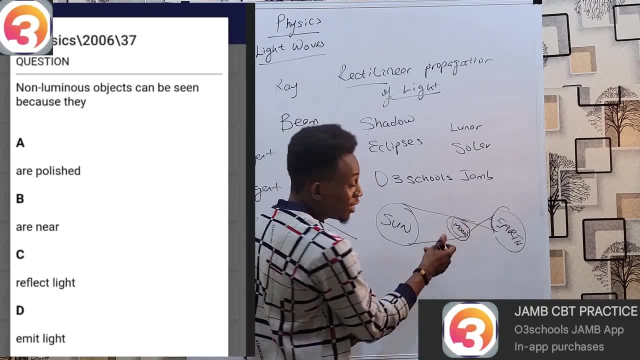 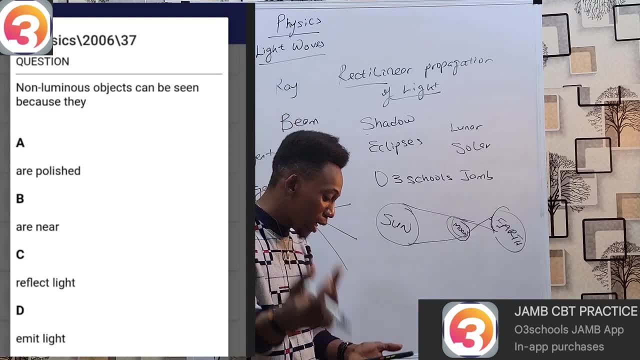 of that one more time is the moon. for that reason, you can try see these bodies, because they reflect light which has already been produced and it bounces back to the eye of the observer and for that reason you can see them, which means, in this case, our answer. 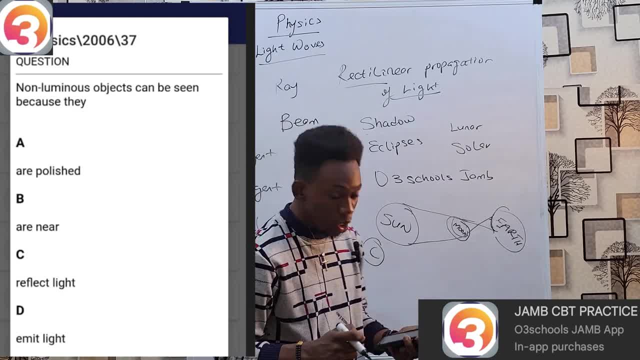 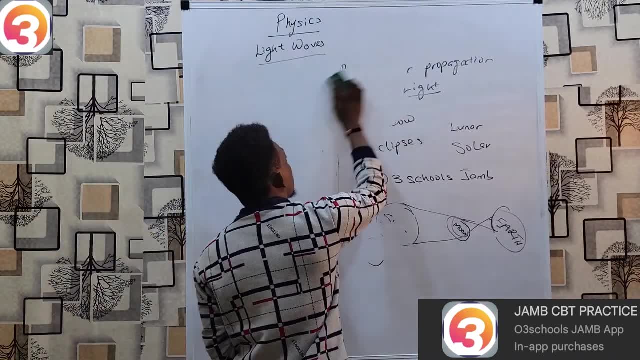 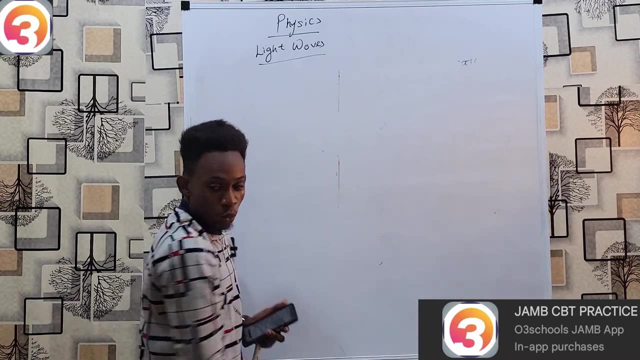 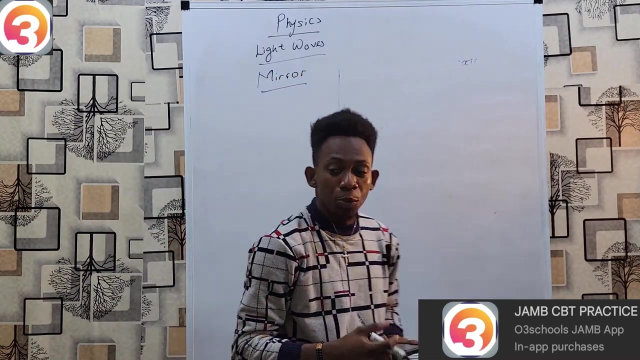 is c. you can see that in your app. okay, that's good. and from this point we shall move on to something of immense consequence all of us, especially the girls- which is the mirror. we overuse mirrors in our daily lives. what is a mirror? in essence, a mirror is simply a piece of glass. 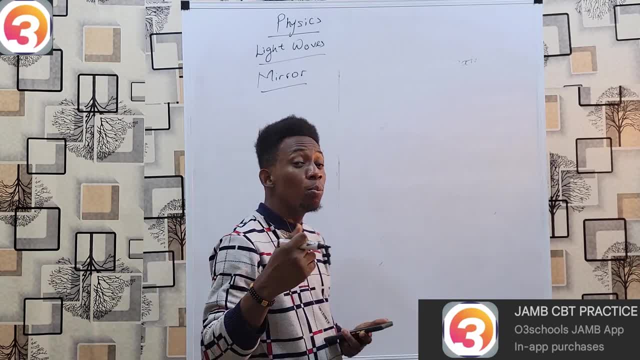 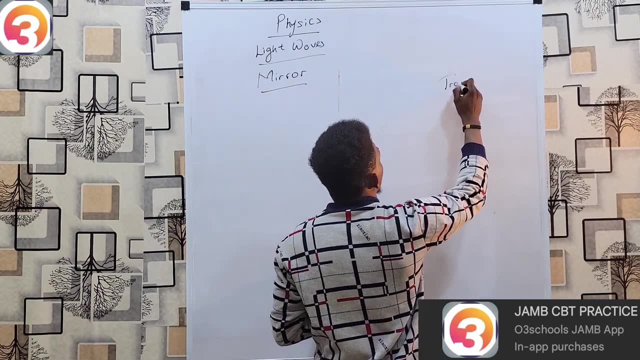 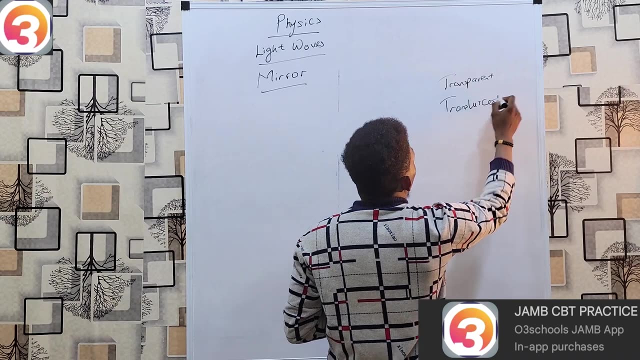 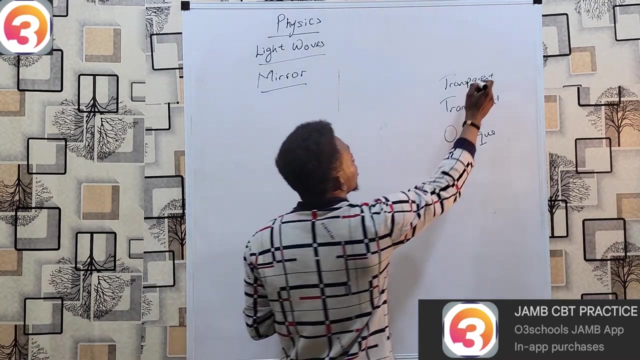 which has been coated on one side and, as a result of that, it's able to bounce light back. because, as you know, in life there are three types of objects. we have the transparent, the translucent and the opaque. transparent objects: they simply allow light to pass through easily, so 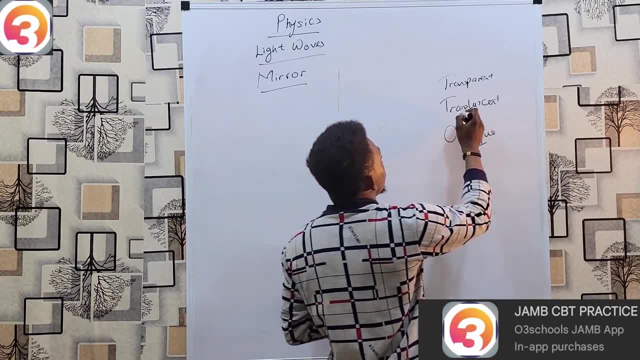 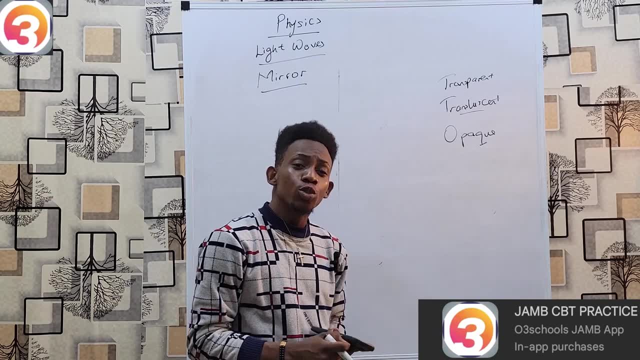 you can see through a transparent object. a translucent object, on the other hand, allows light to pass through partially, so you can kind of see through them. but I've tried to look through some sort of things. you may be able to see what is in front of you, but not really clear while opaque. 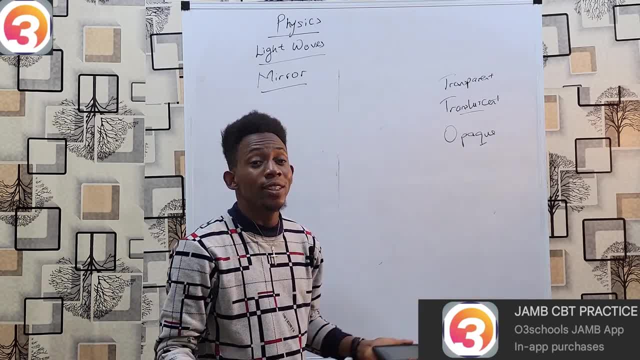 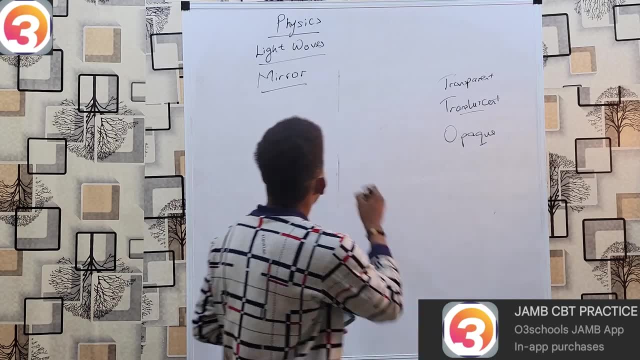 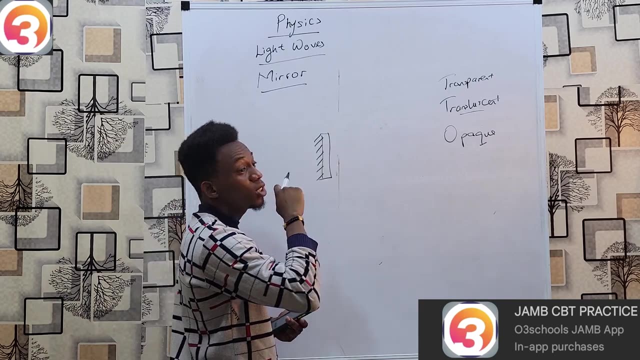 objects, no light pass through at all. your wall is a good example. you can't see through a wall. now, as you aware, your glass is usually translucent, but on coating one of the surface of the glass, usually with a seething gray material, your glass becomes reflective, so any light that goes into it. 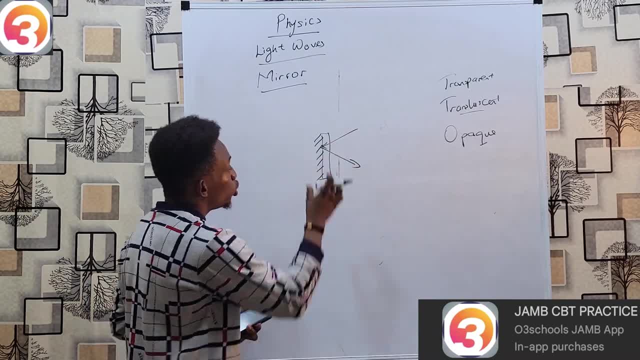 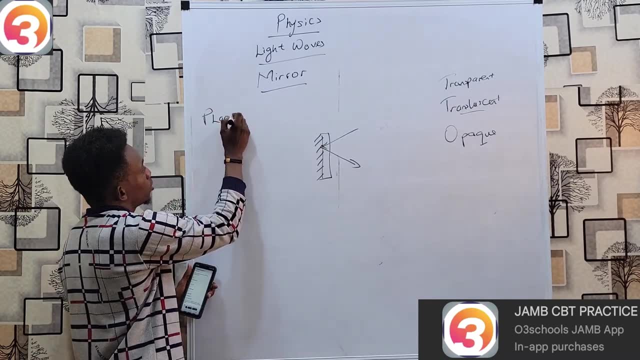 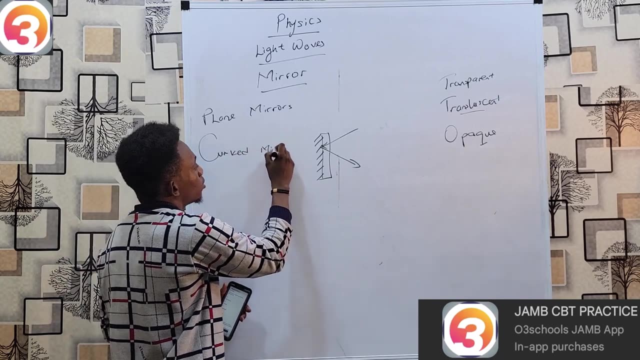 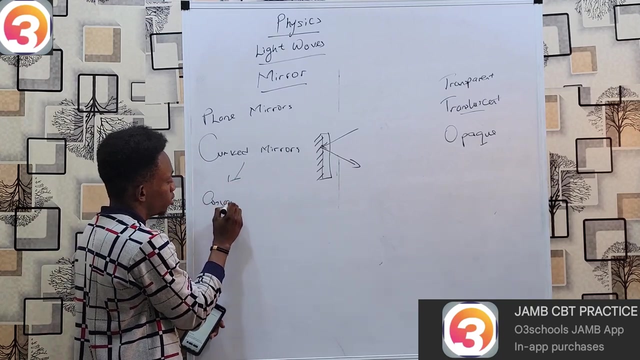 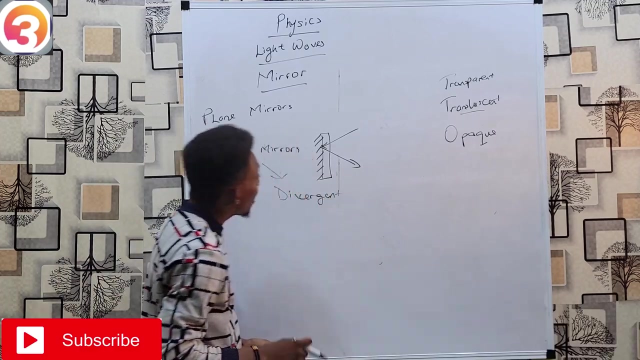 bounces back. I want to do this with: produced a mirror. okay, our mirrors are of two types. generally, we have clean mirrors and we have cold mirrors, your cameras also, before that breakdown in so convergent and divergence. but for now, we shall be starting our focus on plain mirrors. now, how do you produce plain mirrors? 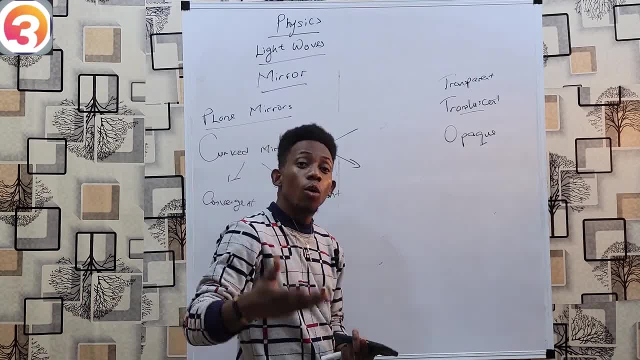 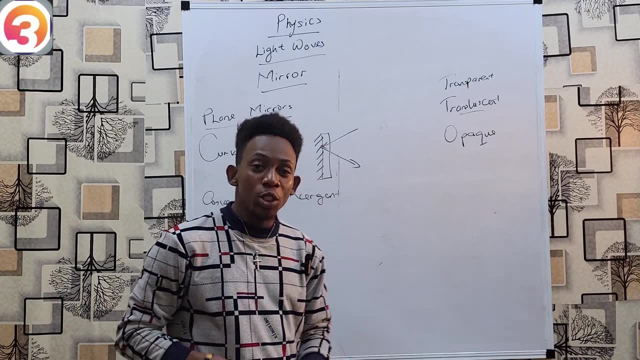 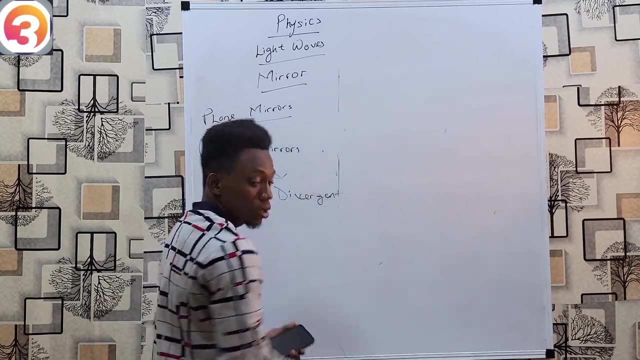 cameras are gotten from straight pieces of glass, unlike a cold moisture. I bought it from cold pieces of glass. your clean mirrors are perfectly straight and, as a result, the images they produce have some special properties. number one: the image produced by a plain mirror are always the same size as the. 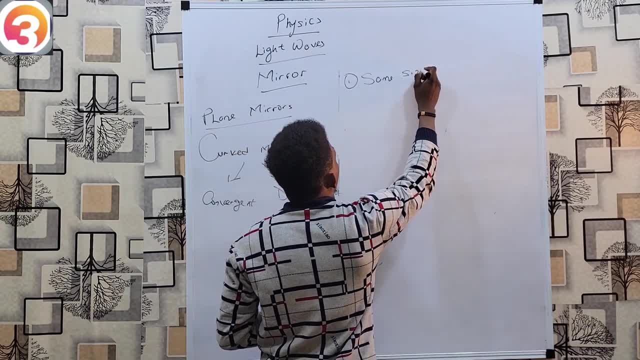 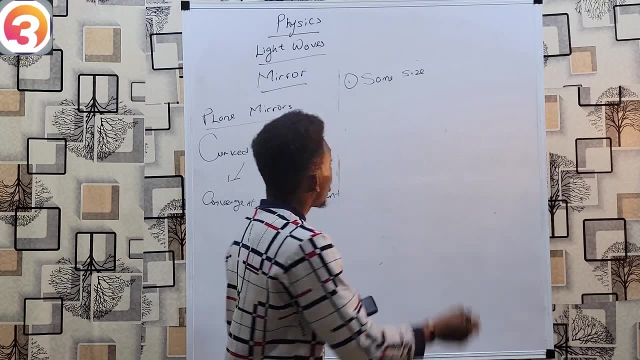 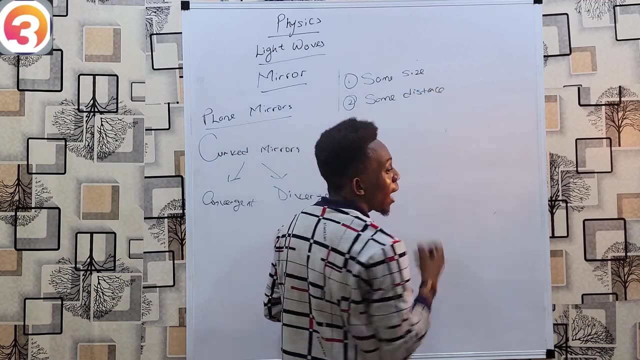 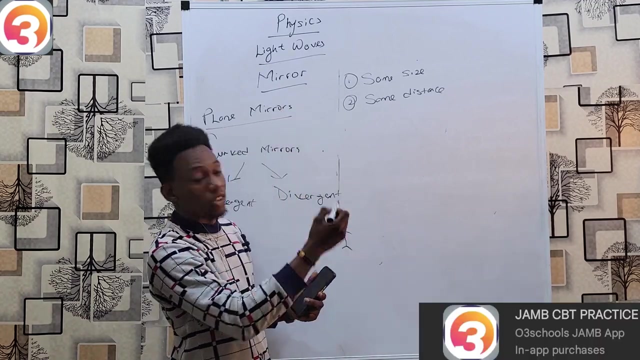 objects, never bigger, never smaller. also, the image they produce is at the same distance in the mirror as object is in front of the mirror. what that simply means is that if I also have a man- let's take this as a man standing five centimeters in front of the mirror. 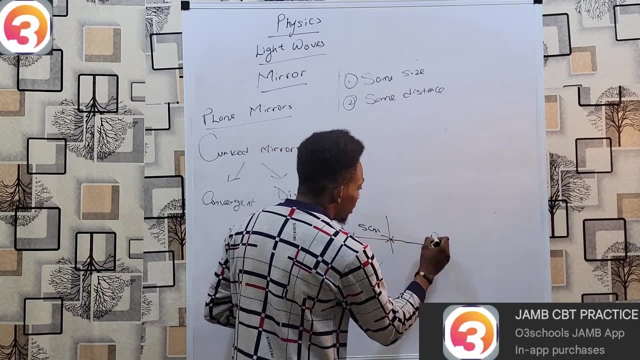 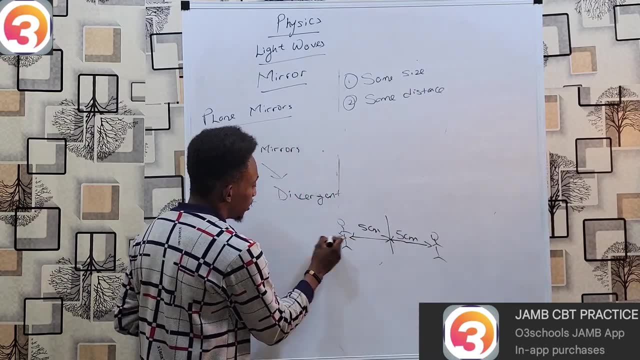 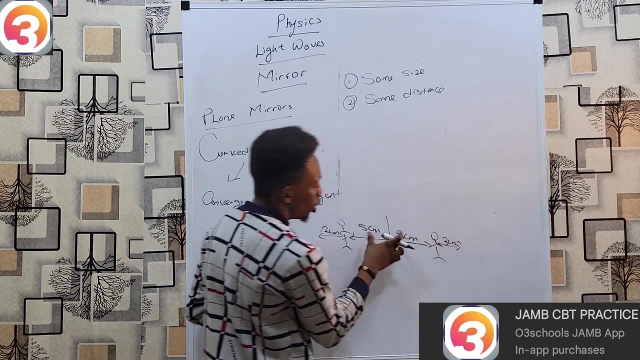 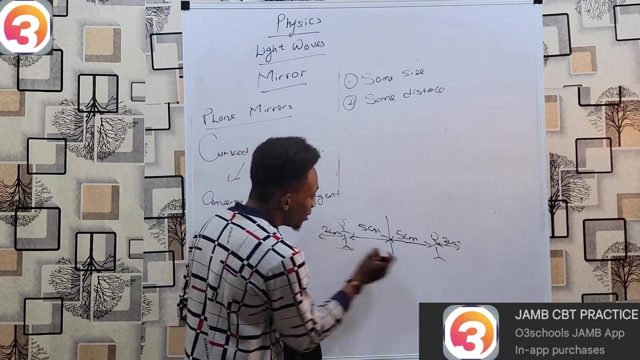 his image on the other side of the mirror shall also be at a distance of five centimeters. if he moves back a further two centimeters, the image will move inwards a further two centimeters. so they shall still be at seven. seven, so that's what it tells us at the image, while the same size will also be at the same distance. 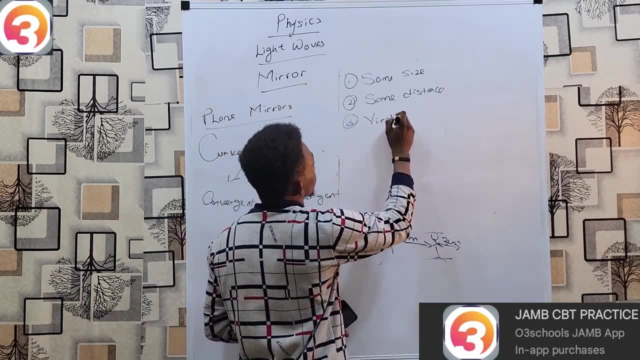 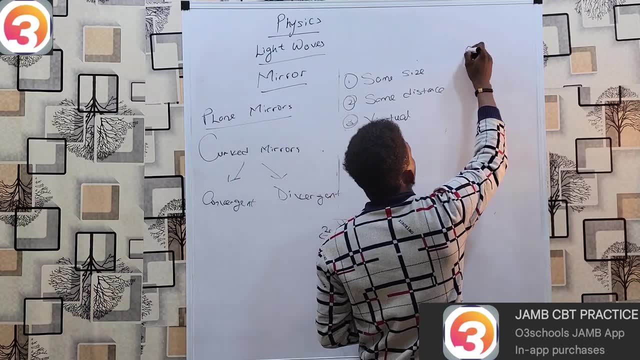 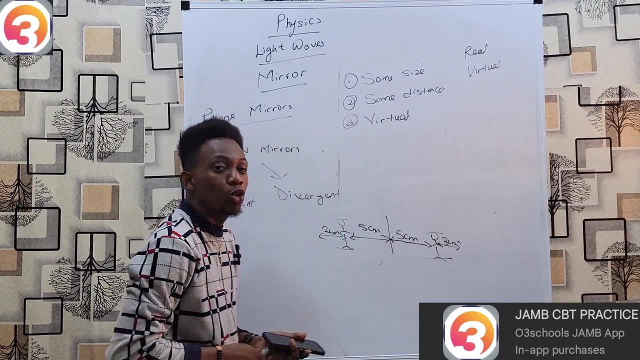 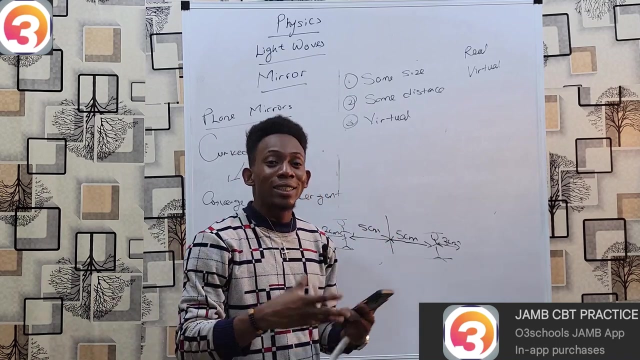 now? thirdly, this image is virtual. now, what does a virtual image mean? we have that of images. images can either be real or virtual. they will image that image that can be captured on the screen. what that simply means is: um, if you are to reflect this image onto a photographic plate, you should actually take a picture that you 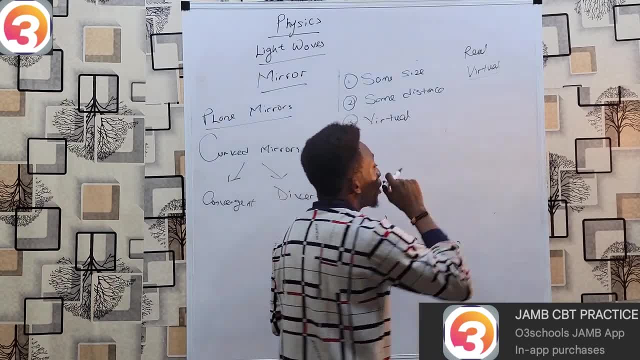 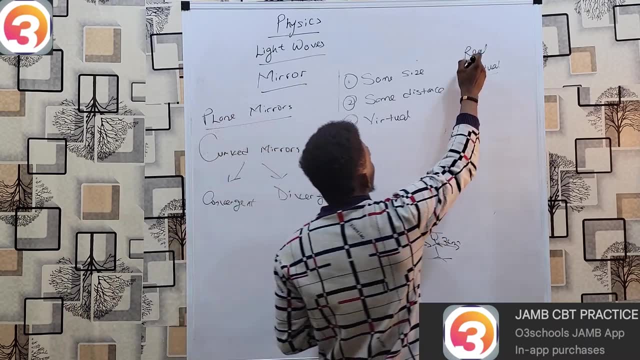 can share both. with a virtual image, you cannot try to keep it. if you put on a photographic plate, take it. if you put on a photographic film, all you may get is nothing. you cannot try to see it. that's the biggest difference between real and virtual images. so the one you get from your mirror is 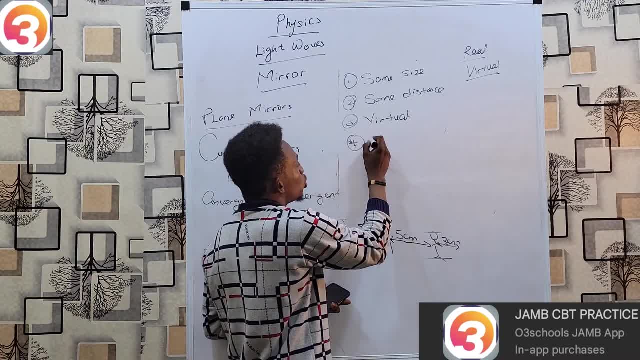 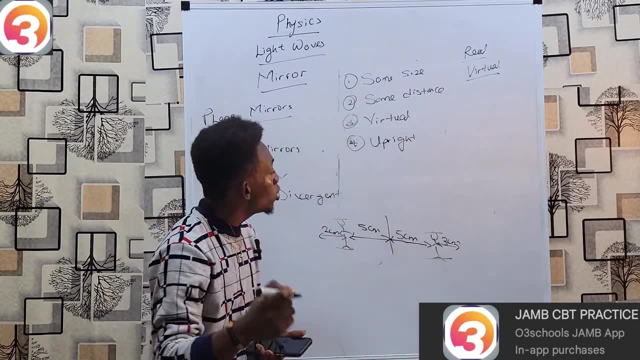 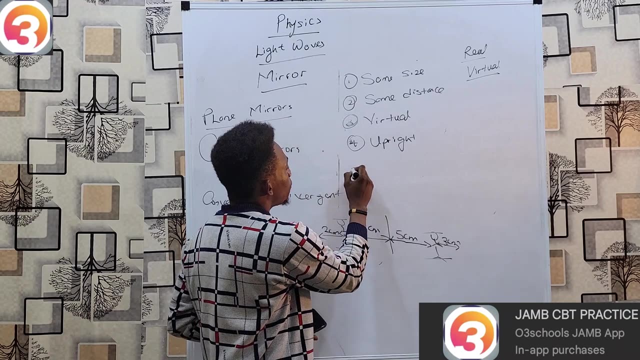 virtual. and fourthly, this image is going to be upright. if you are standing still, the image you see of yourself in your mirror will also be standing. your image will not be upside down. it will definitely be right side up, just as you are. but the fifth one is a little bit tricky. 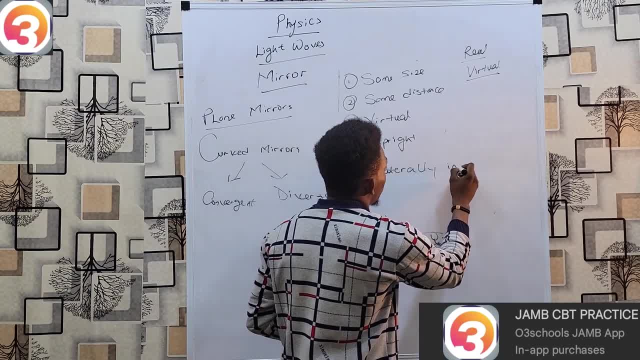 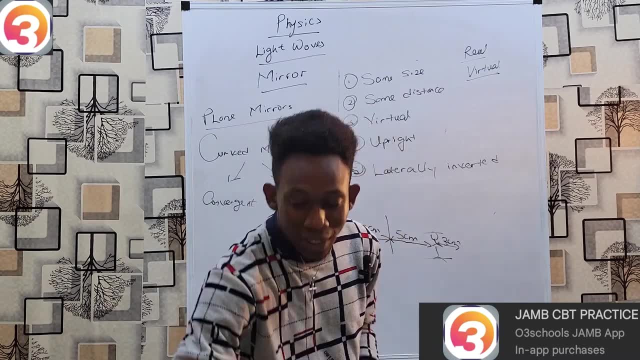 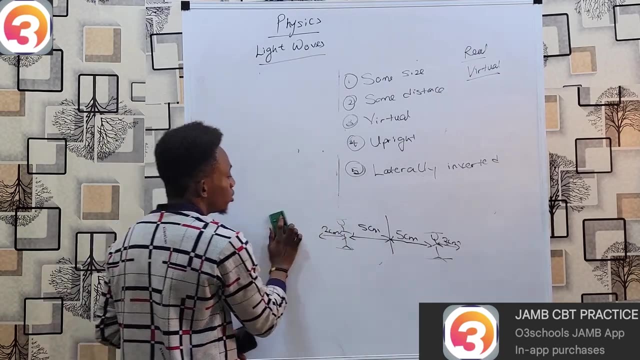 this one says that the image will be laterally inverted. lateral inversion: what it means is that the image is spun around its axis of symmetry, implying that if you have to try looking at writing in a plain mirror, there shall be a bit of confusion. you can try this at your. 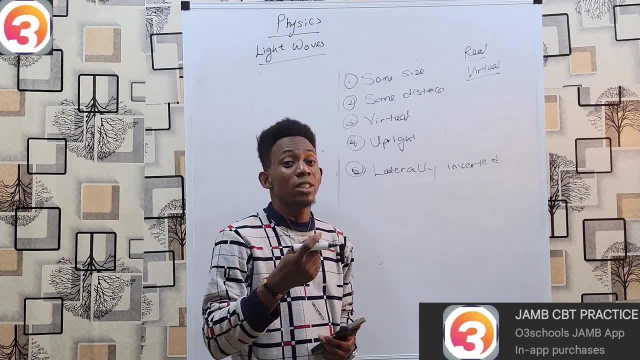 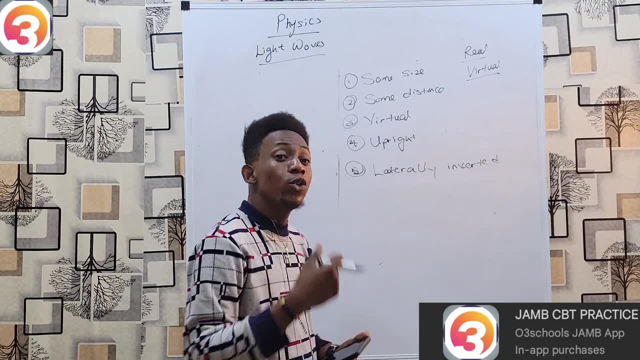 homes. take a book, start with a photo of your house and start with a photo of your house mirror and try reading it. your image while also the book would not really make much sense if you also stand for the mirror and raise up your right hand. the image you see in the mirror. 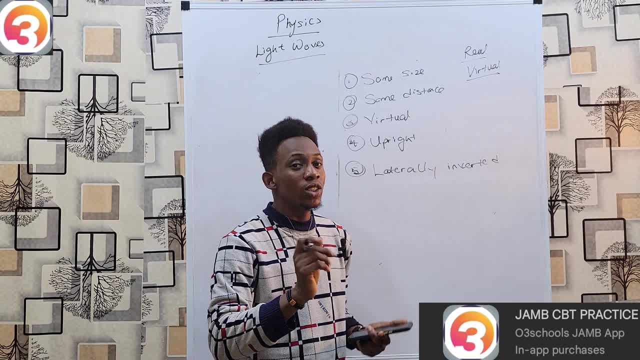 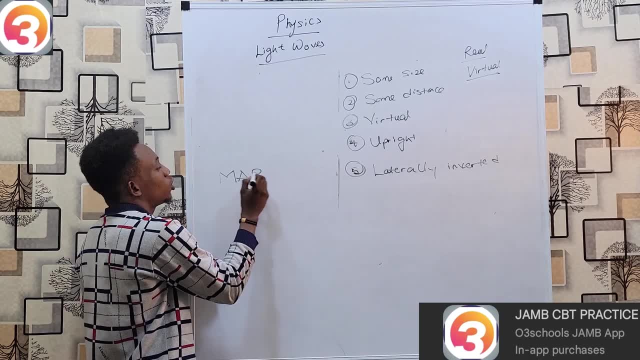 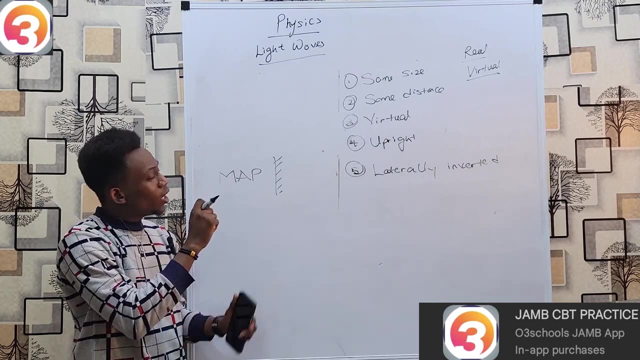 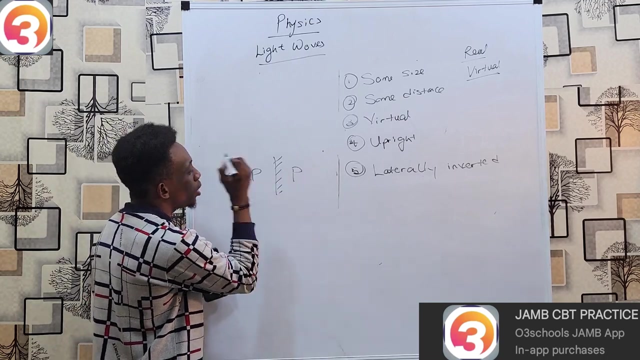 will be raising up its left hand, not its right hand. so you notice, left and right are kind of switched. that means, if i also take this map so a mirror, what i will see in this mirror will no longer quite be mapped. instead, everything gets spun left to right. so my p will confess, but instead of appearing as p, 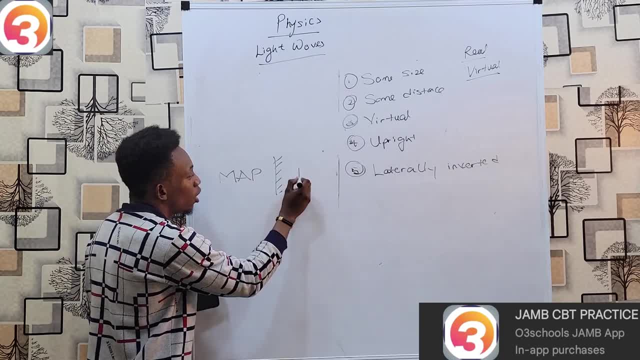 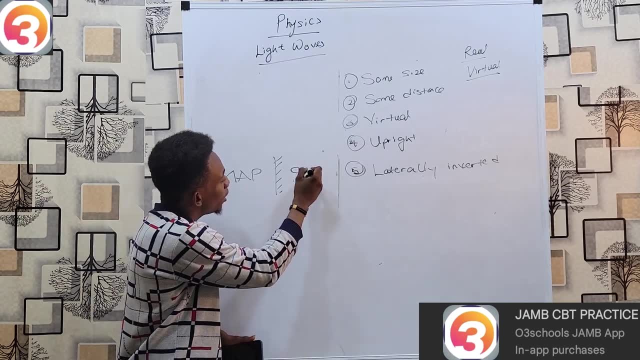 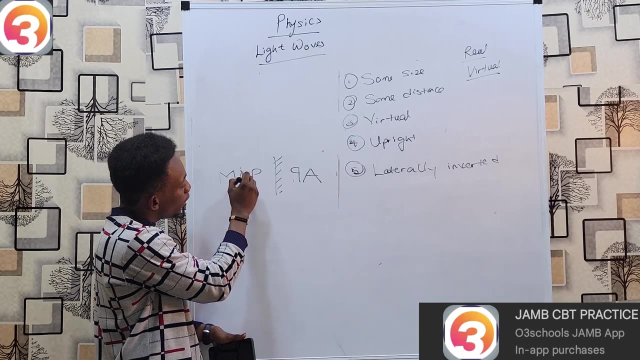 this curve on your p will go the other way, instead making it look more like 9, but on the other hand, a. if you look at a, no matter how i switch a, A remains A, because this line of symmetry is parallel to the mirror. so every image. 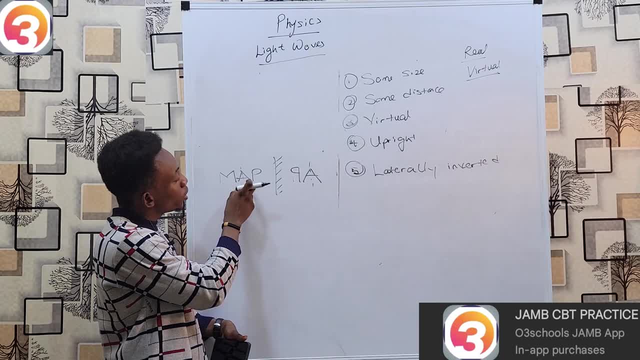 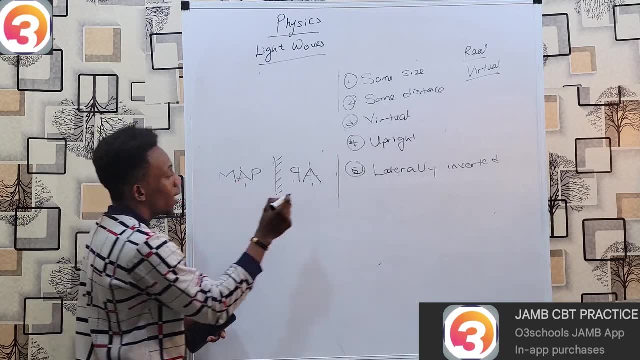 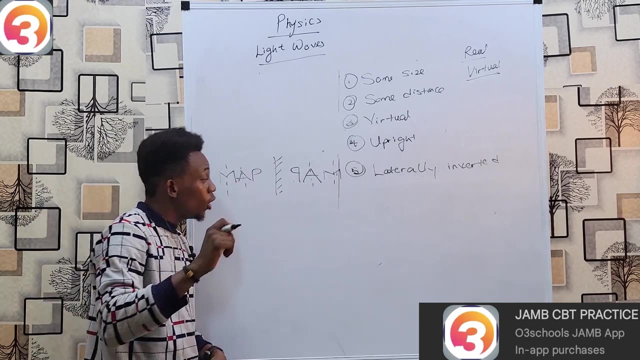 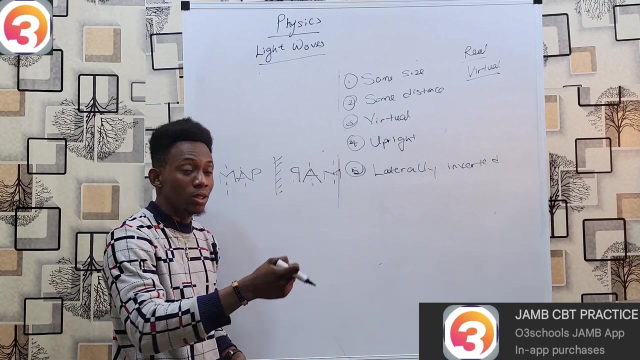 you see, in symmetry is parallel to the mirror. the mirror remains the same, but if it is not, it gets distorted. so a is a, m would also be m, because the line of symmetry is also parallel to the mirror. it is that simple. so every image gets spun around. those whose line of symmetry is not prior to the mirror get distorted, but those that 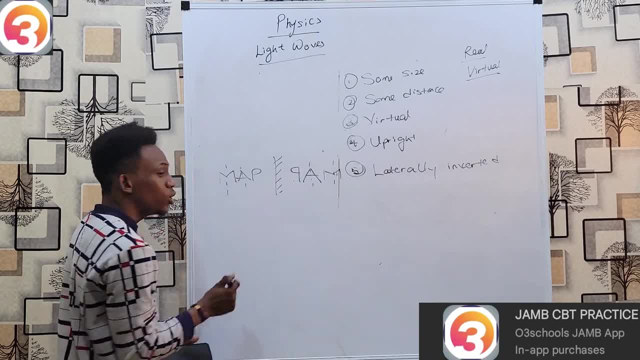 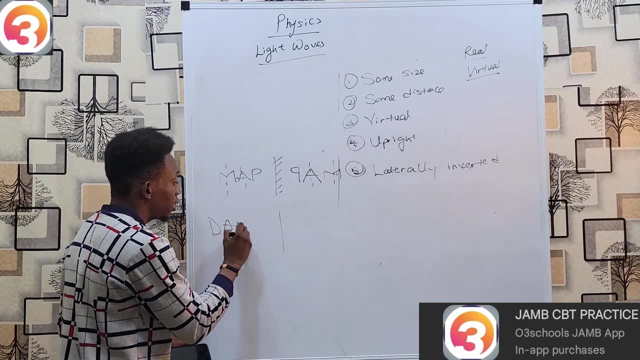 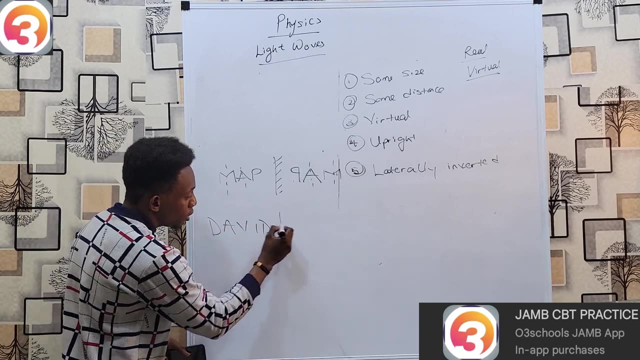 have. symmetry is prior to the mirror remains the same. this is one example. we could try a different word. let's say um david as a name. to look at david. this d doesn't have the line of symmetry parallel to the mirror. therefore d sort of calls around and looks different, but letter i is parallel. 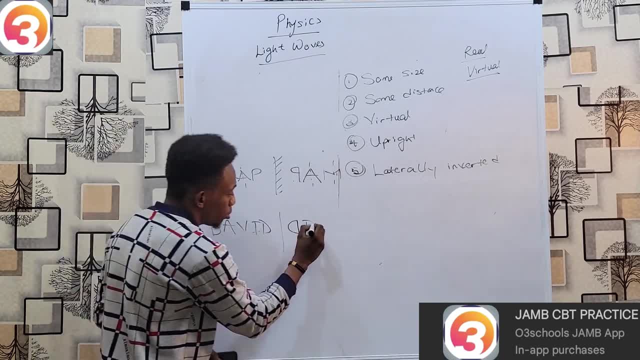 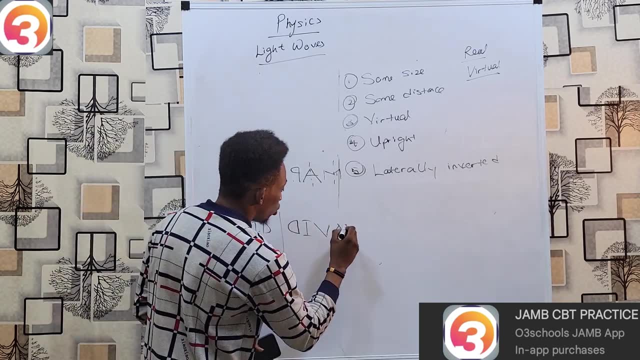 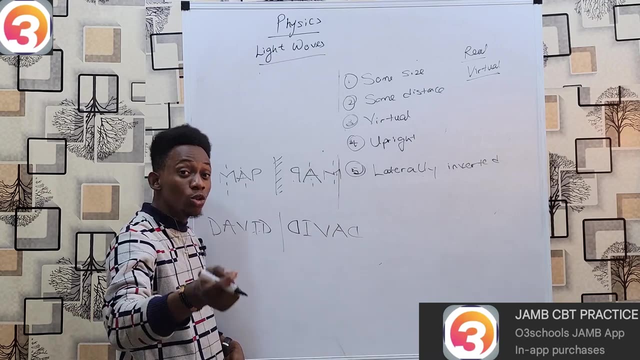 so i remains, i letter. v is parallel remains the same. a is parallel remains the same, but our d will also spin. so if you're to take this, if you're to write this in your notes- a good way to know when you're correct- say this is your writing and look at this in the mirror, when the mirror switches it back, for 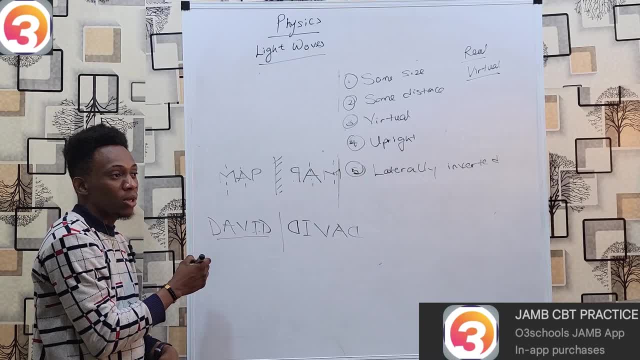 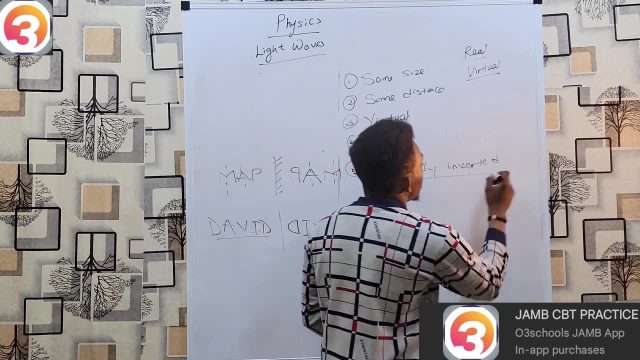 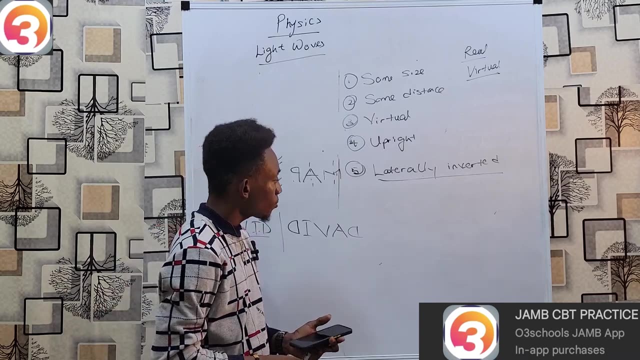 you, you shall realize that you now have something perfectly normal. but if you take the number one to the mirror, the mirror makes it distorted and that's referred to as lateral inversion. okay, and that is the property of your plane mirror. that's what i'm talking about. 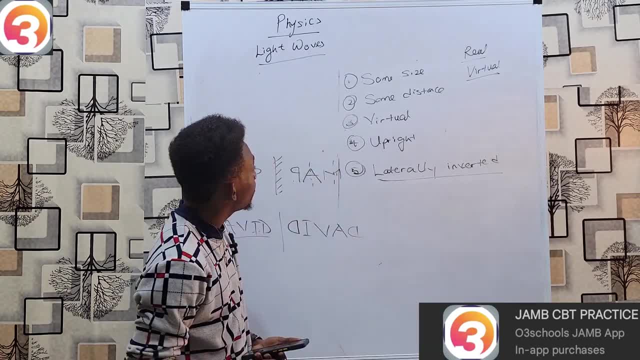 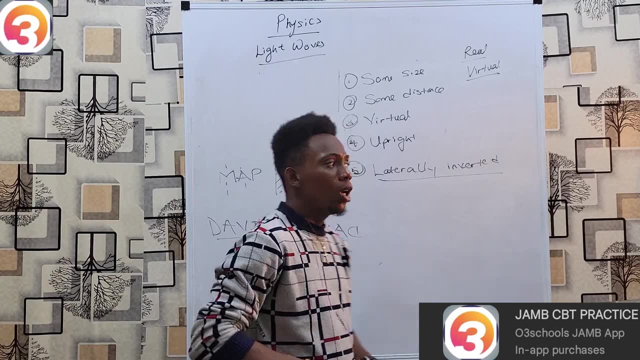 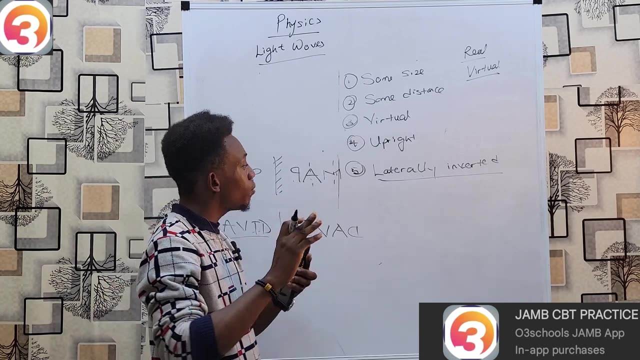 um, all right. so that's that for our plane mirrors and the portrait of the image. now, however, this plane euros can still do some other things. if you've ever stood um at some mirrors that are called- and when i say cough and i don't mean cold- 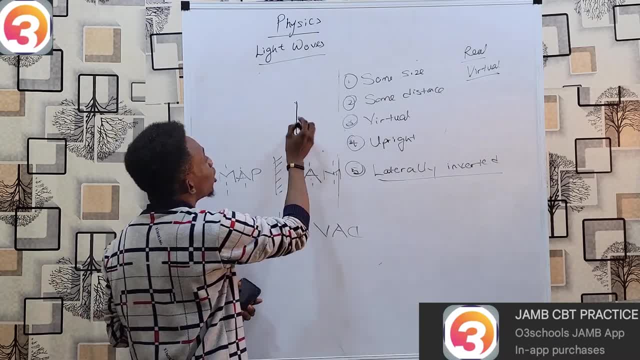 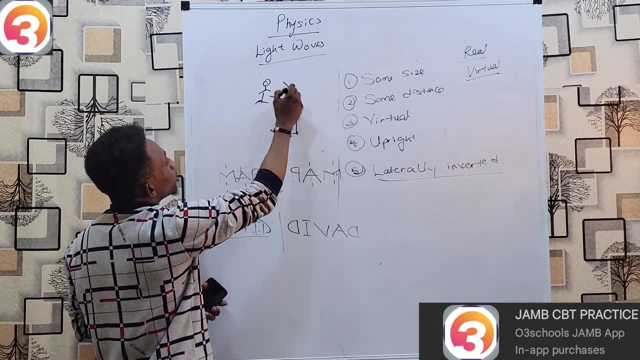 sense, that may mean two plain mirrors joined together at an angle- something like this. do you? So you now have you standing right here in the center and looking this way. If you've ever observed that, you realize that you can see more than one image at times. 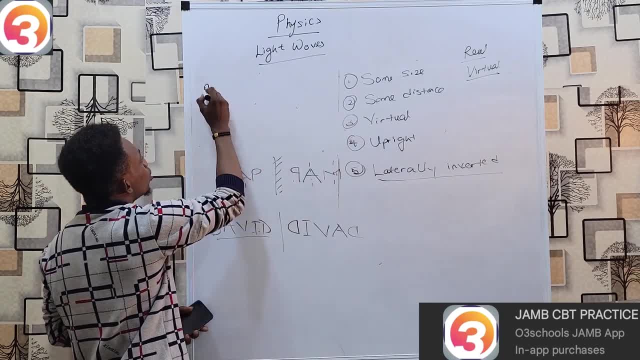 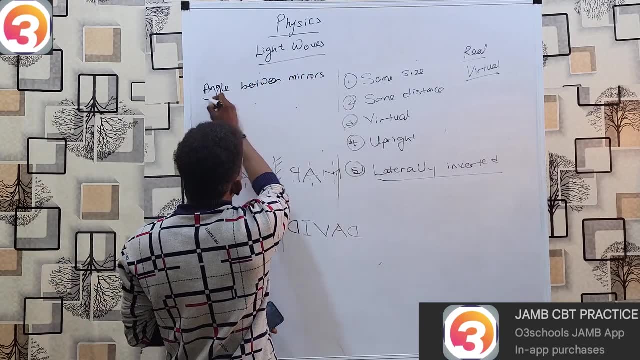 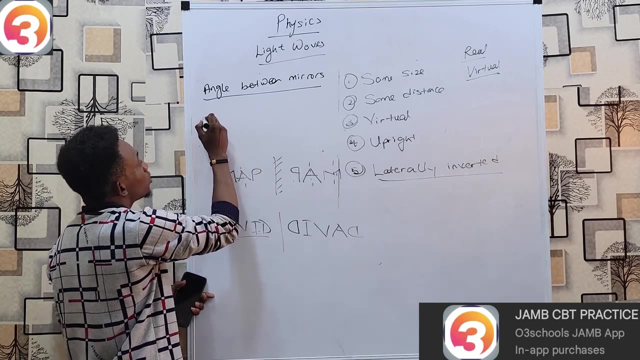 And that is a property we get based on the angle between the mirrors. So if you have any two mirrors joined together, the number of images you see depends on the angle between the two mirrors. And to get that you turn a general formula. 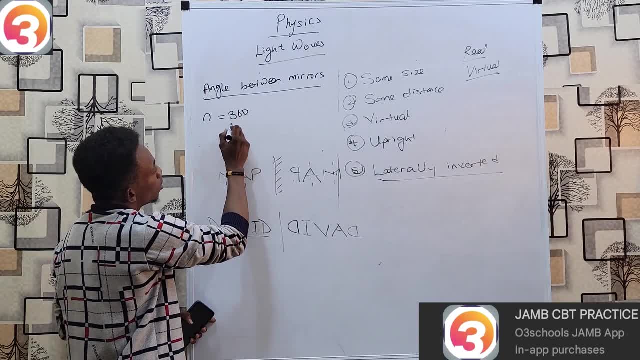 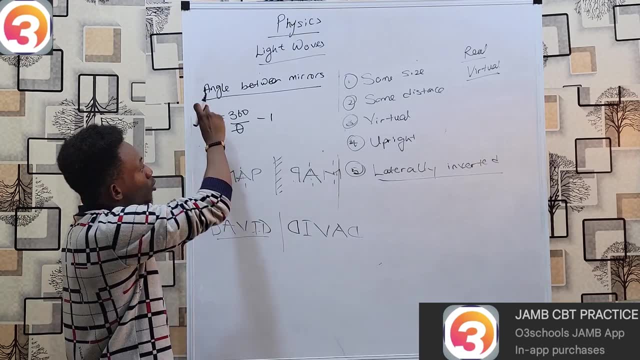 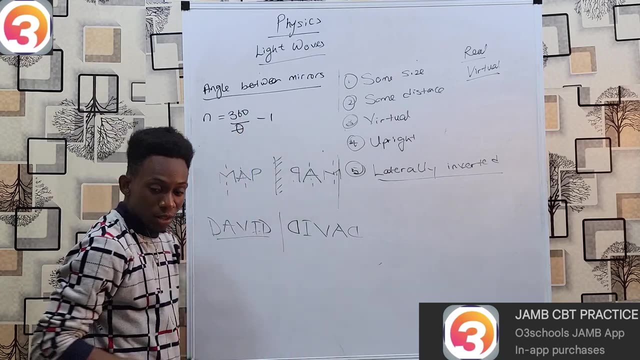 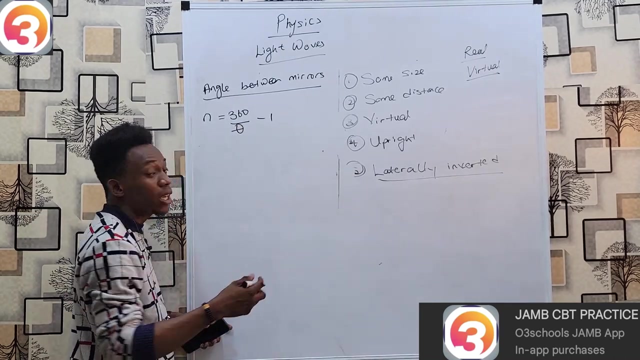 which is that number of images equals to 360 over the angle between the mirrors minus one. That's a formula: Number of images equals 360 divided by the angle between the mirrors minus one. That means that if, for example, we're having the angle between the mirrors being 90 degrees, 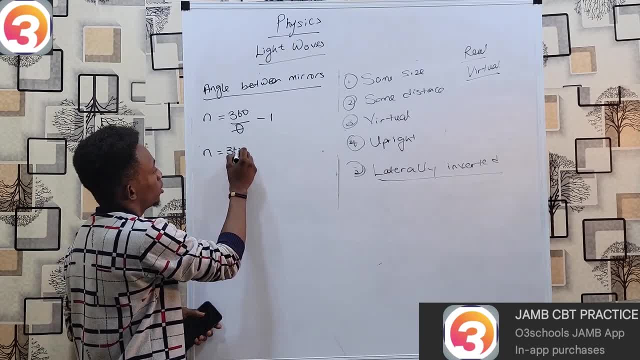 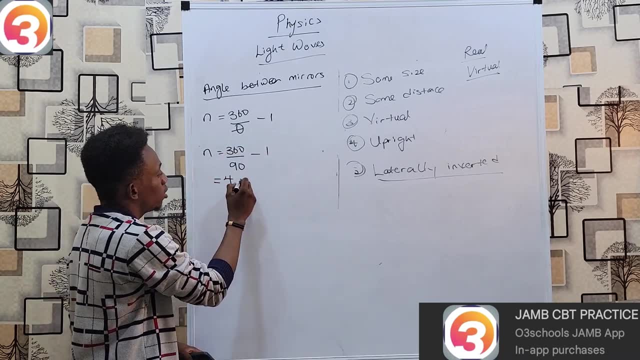 as is common, our number of images becomes 360 over 90 degrees. So that means 360 over 90 minus one. 360 over 90 is four. four minus one is three. That means if we were to stand between two mirrors. 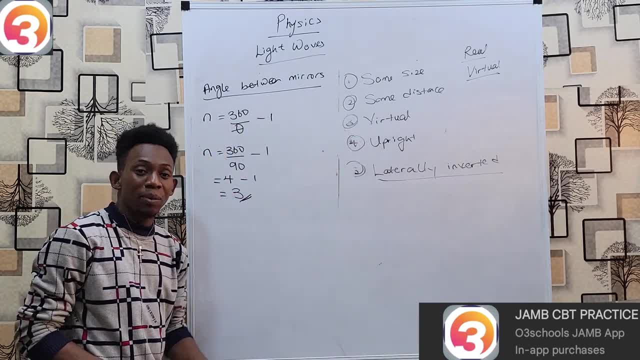 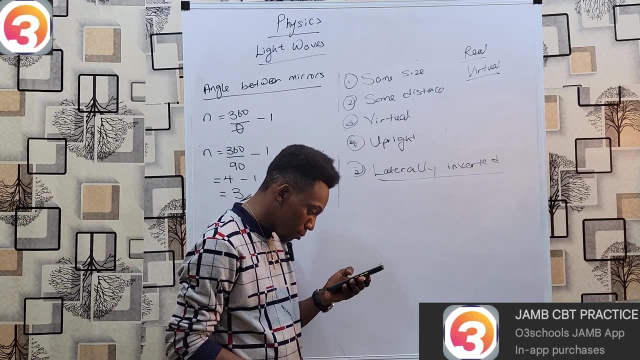 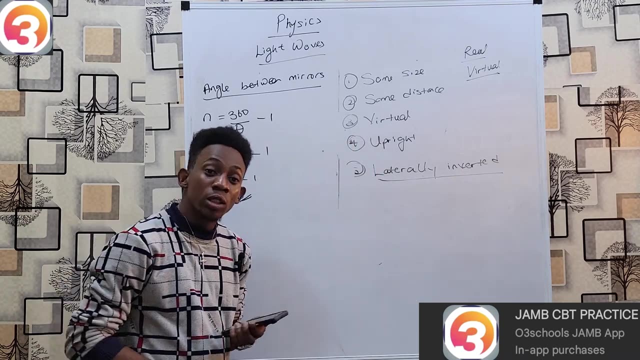 inclined at 90 degrees to each other, we shall be able to observe three different images, And with that we head over to our app to answer a question on this subtopic. Now, this question is quite simple. This question states if an object is placed between two parallel plain mirrors. 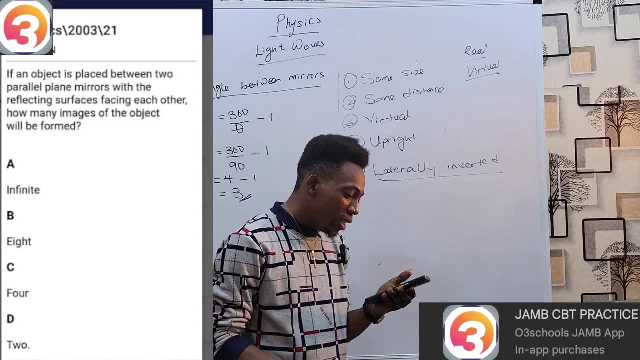 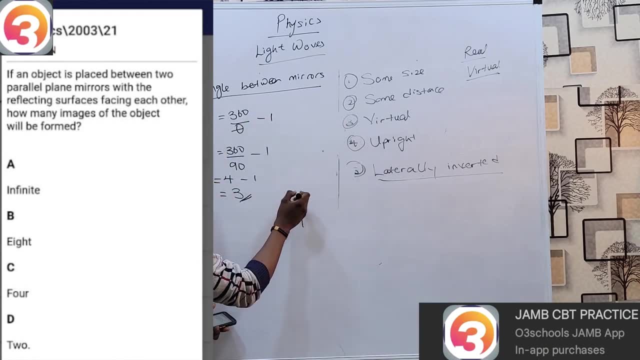 with the reflected surfaces facing each other, how many images of the objects will be formed? Now, in this case, it's more like this: that we have a mirror here and another mirror here, and the person is standing right here Now with this. if you look at this, 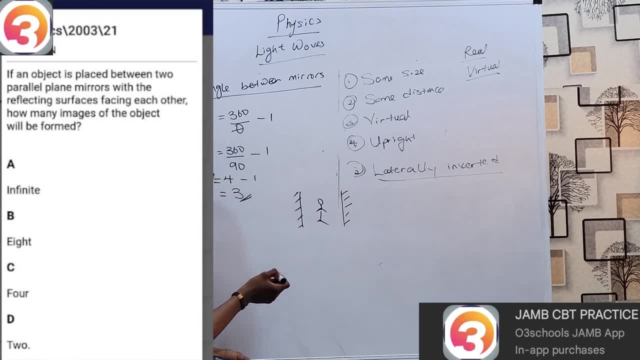 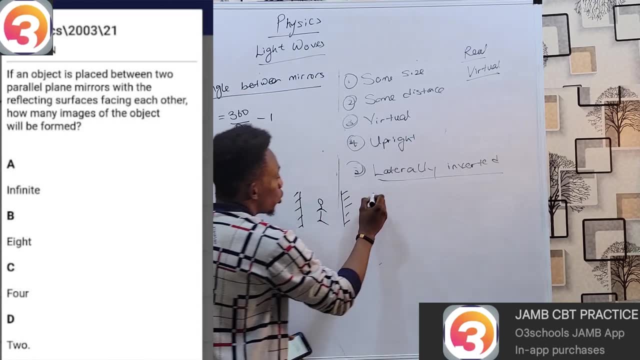 what is the angle between these two mirrors? That is the first trick of the question. If you have to look at this, they are not toned at all, which means that my angle must be zero degrees. So if our angle between the mirrors is zero, 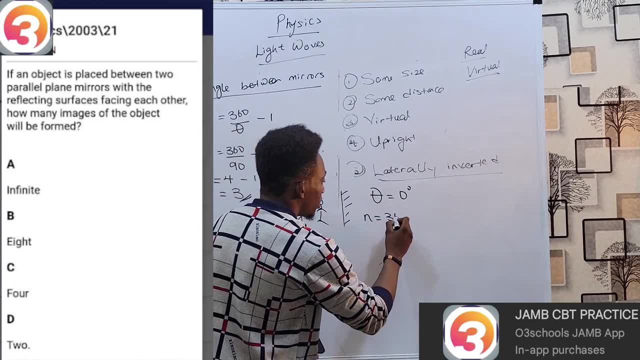 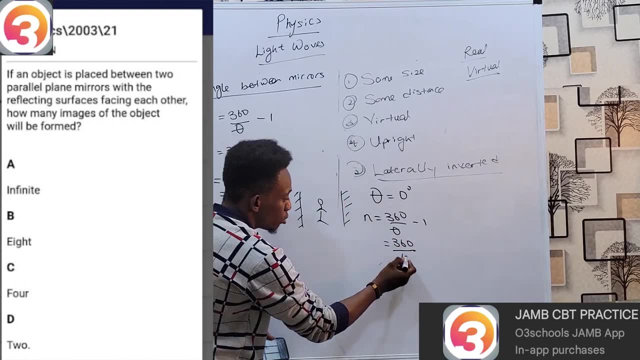 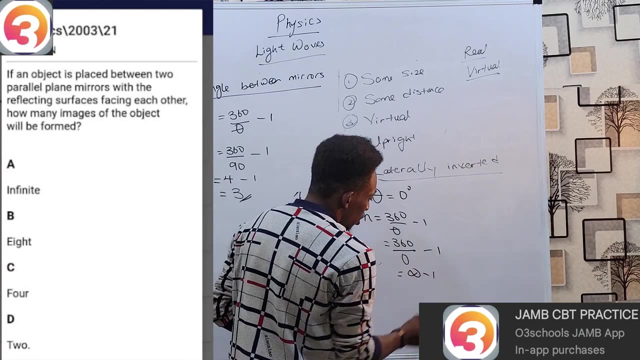 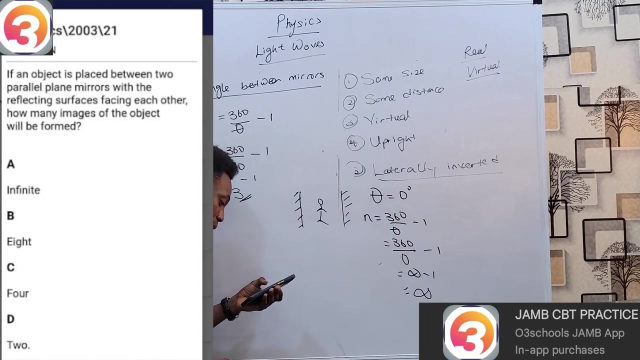 applying my formula one more time: n equals to 360 over theta minus one. that would be 360 over zero minus one And, as you're aware, anything divided by zero is what Infinite. So infinite minus one remains infinite And therefore our answer is A infinite. 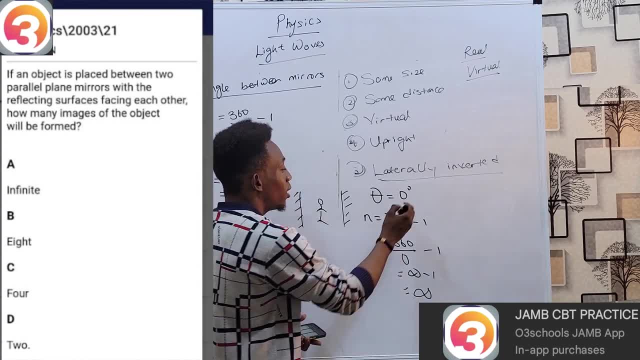 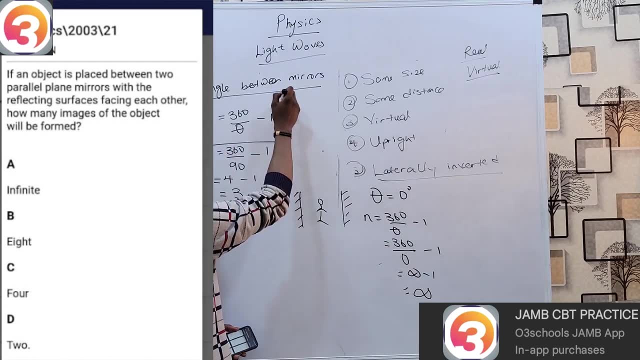 It's that simple. So for these questions, the first thing we must identify is the angle between the mirrors. Once you know that, to get your number of images, simply apply your formula, And that is how we deal with angle between mirrors. 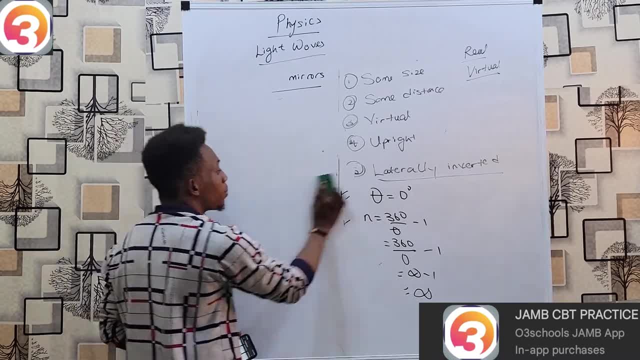 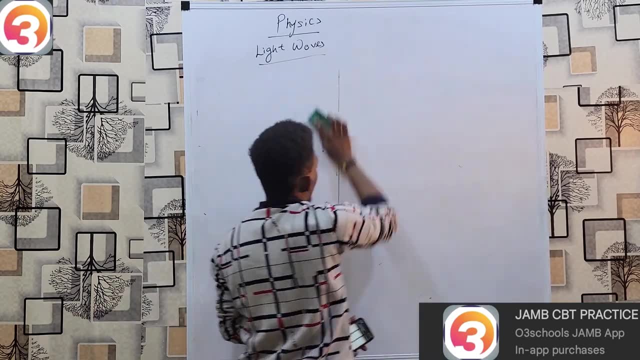 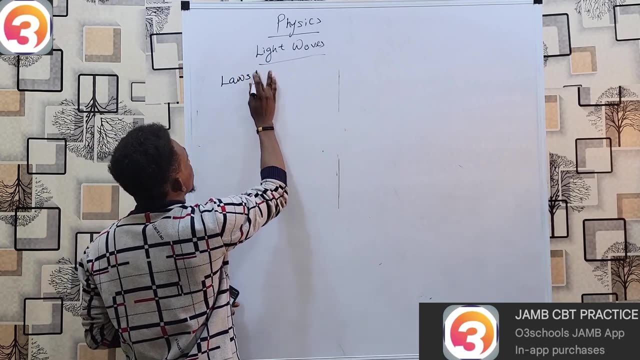 Now we shall be looking at this question. It's worth something less. Still on that, clear mirrors, we shall be wondering what happens if I rotate my mirror. Here's the thing. On the clear mirrors, there are two laws that govern how the image gets reflected. 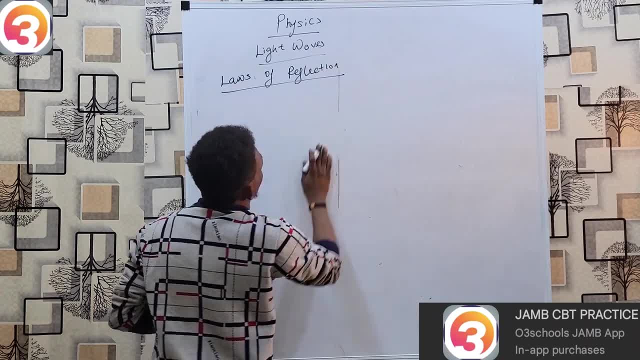 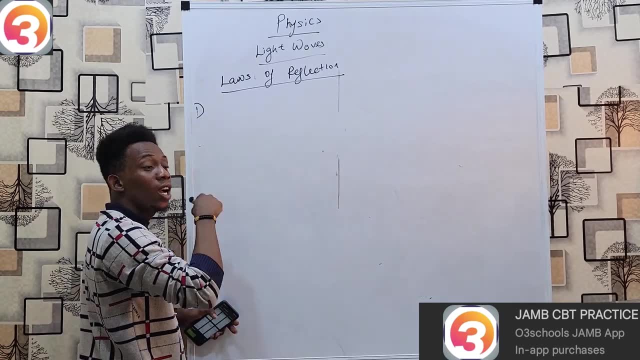 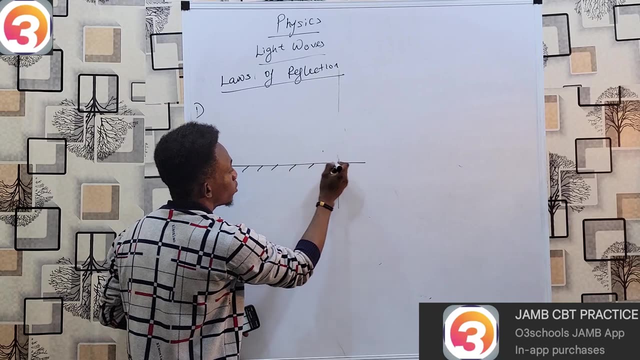 The laws of reflection. Now, the first law of reflection simply states that the incident angle, the reflected angle and the normal all lie on the same plane. That means, if this was my mirror and I have light incident upon this mirror, 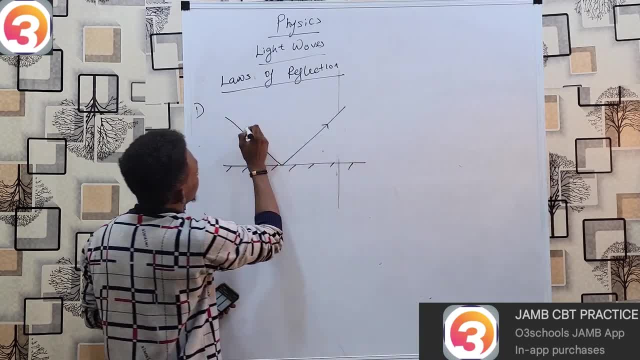 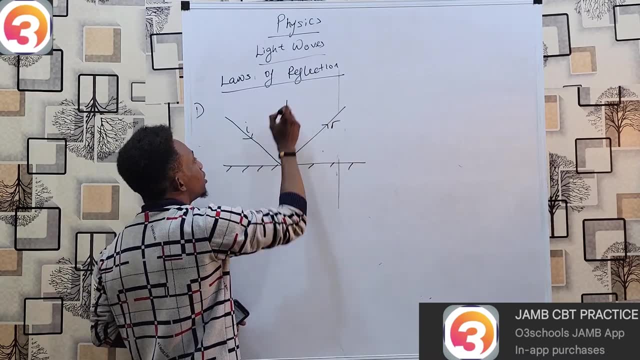 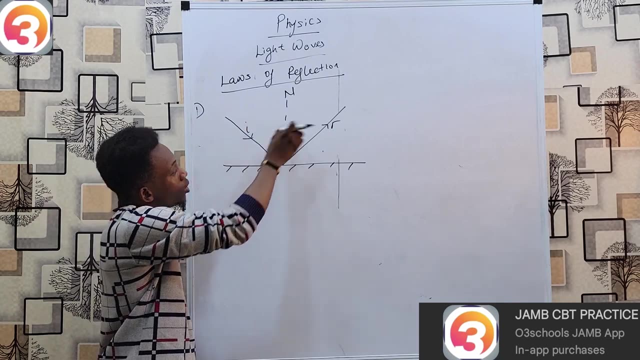 the light is going to obviously get reflected. This is incident ray, reflected ray- And then a line drawn from the mirror at 90 degrees is referred to as the normal. What this law tells us is that this incident angle or this distance ray, the reflected ray- 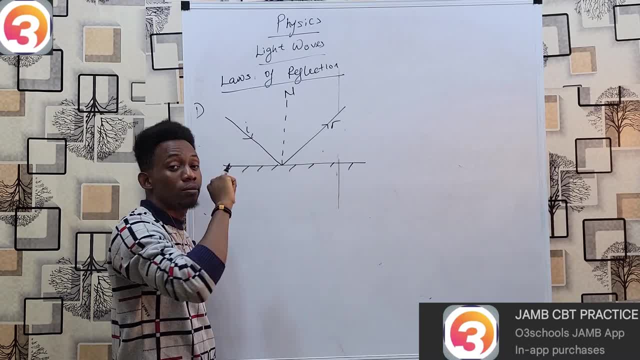 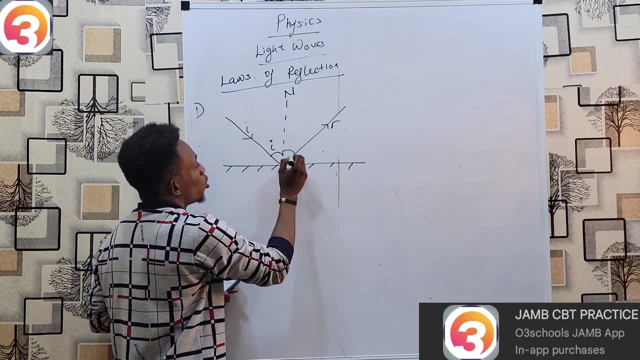 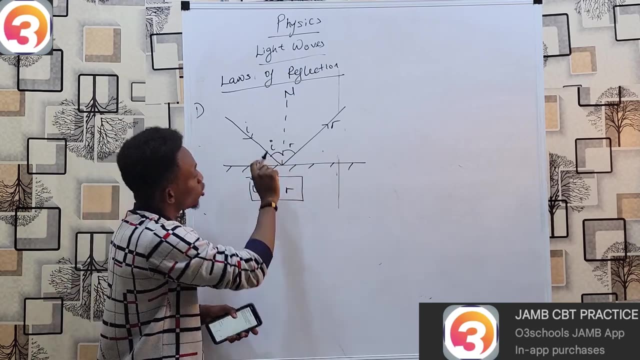 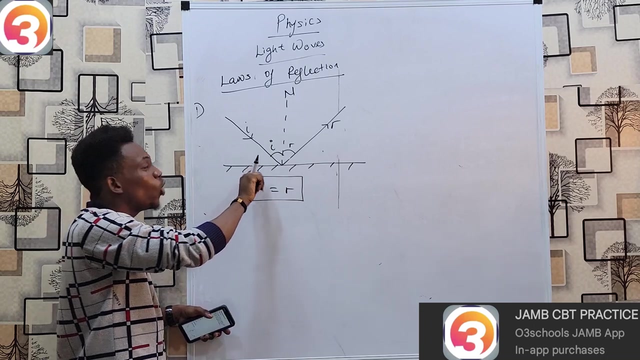 and this normal all exist on the same plane. Why the second law tells us that the angle of incidence is always equal to the angle of reflection. Now, please note: your angle of incidence is always measured from your incident ray to the normal, not your incident ray to the mirror. 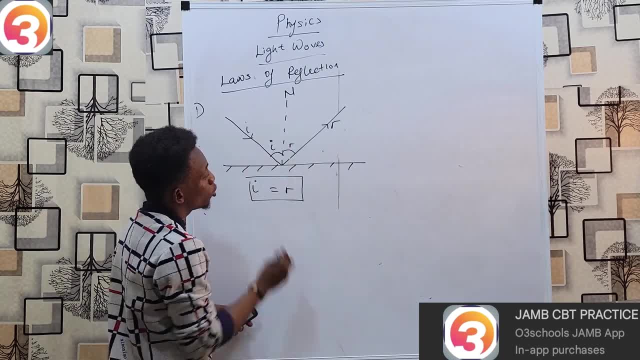 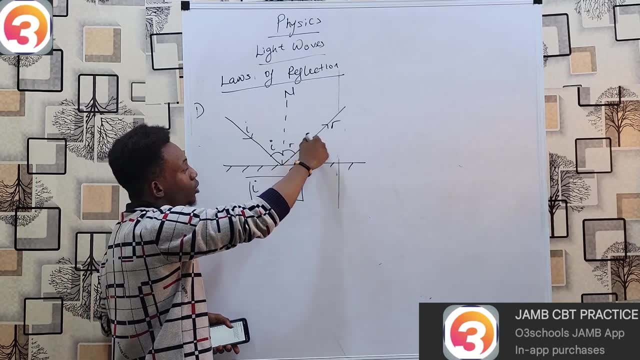 Always from the ray to the normal, while your reflected angle is also measured from the ray to the mirror, to the normal. so in this topic, we do not measure or use the angles we get from the ray to the mirror. instead, we always use the angle from the ray to the normal. 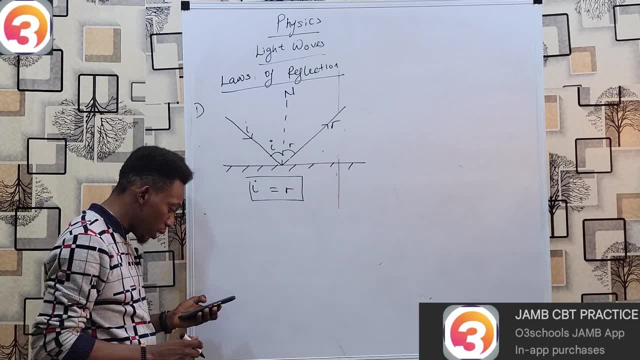 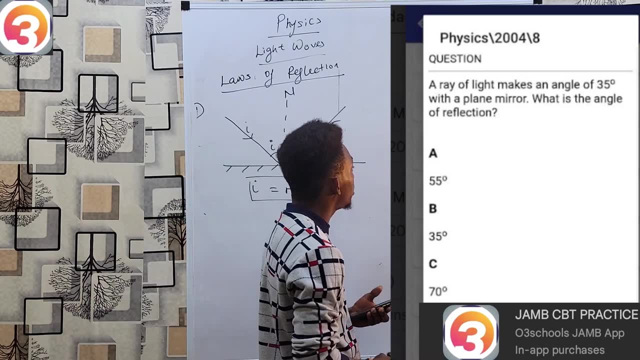 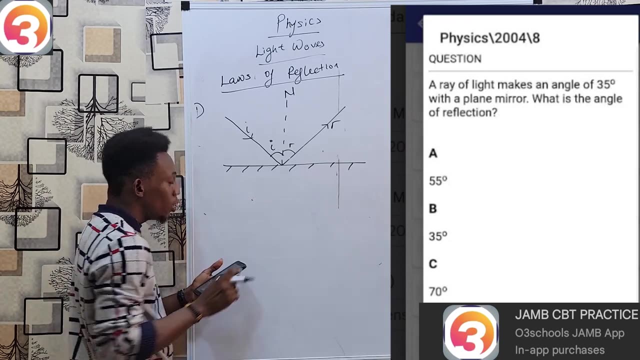 and with that let's take our first question under this path. now. this question says: a ray of light makes an angle of 35 degrees with the plane mirror, which means, if I also use the same diagram to analyze, we have been told that it makes an angle of 35 degrees with a plane mirror, which means: 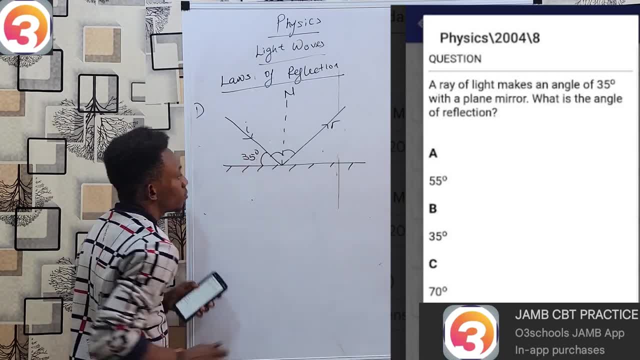 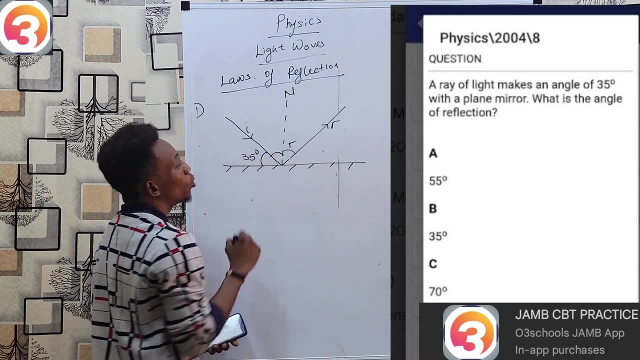 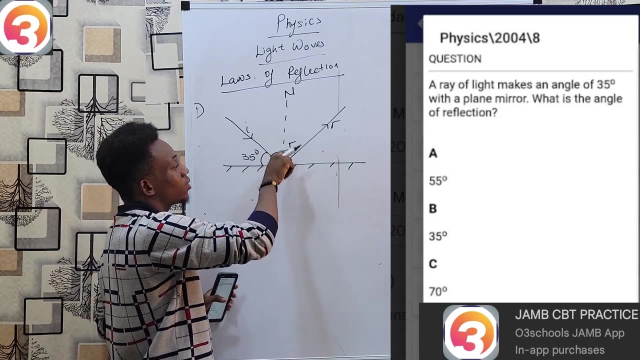 here is 35 degrees, that's our 35, or I've been told to find the angle of reflection. which is this angle? now, as you are aware, before I can go for my angle of reflection, I must first of all find my angle of incidence, and my angle of incidence is: 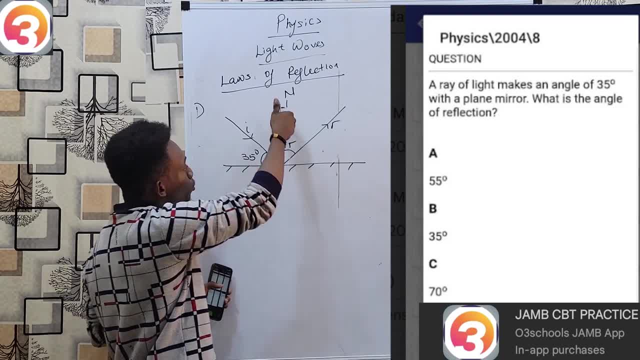 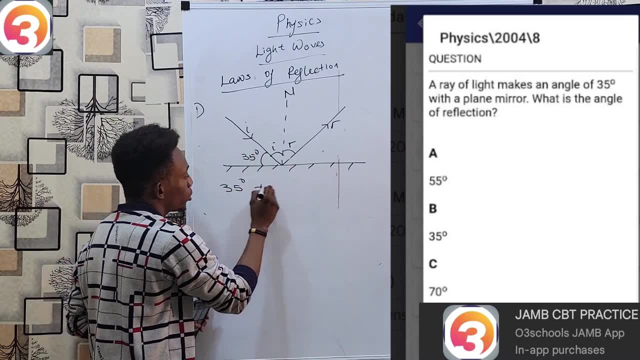 the angle from the ray to the normal. and if you look at this from my perspective and the previous steps now you will see that my angle goes from 35 degrees to 50 degrees, as I can tell, and the angle of incidence is the angle. I must first of all find out the angle of incidence, which is on the right of 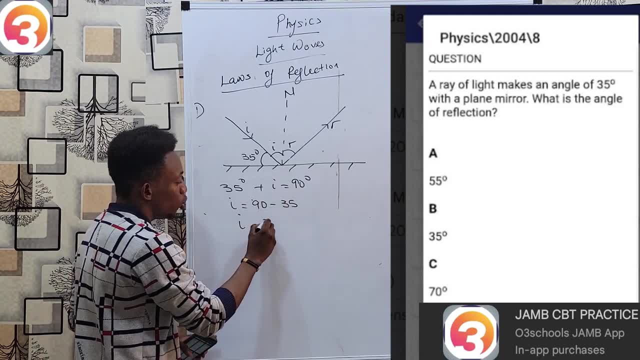 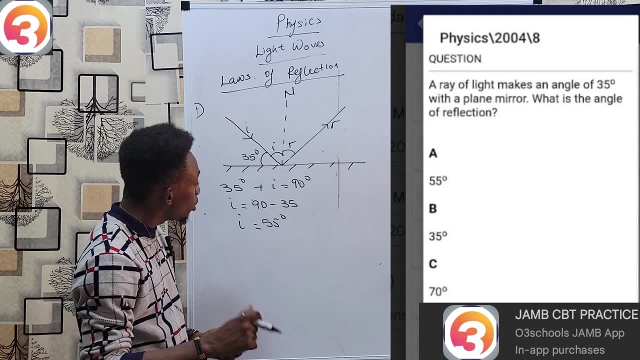 the Earth, but this is the angle that my angle gives us meaning. I am жиз spiritually happy. I know of the length that I have in the universe and that this angle, as I have an angle in my visualization, so 5 degrees length, what can I do so I'm 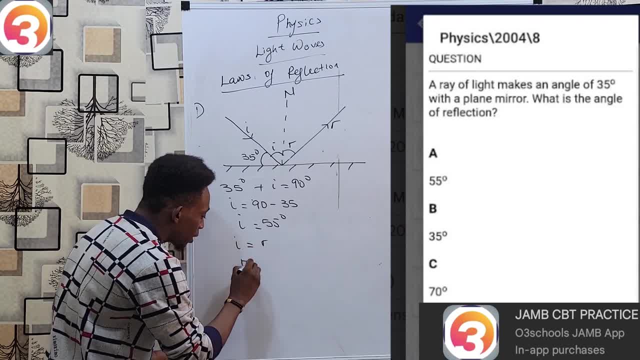 showing this equation: where theximum is the area at which the height of the environment of a worthy solution is 5 degrees, I can use this equation to get results. so this is that first situation: we only emotion. and now, in the second example, whatever occurred, if I content, 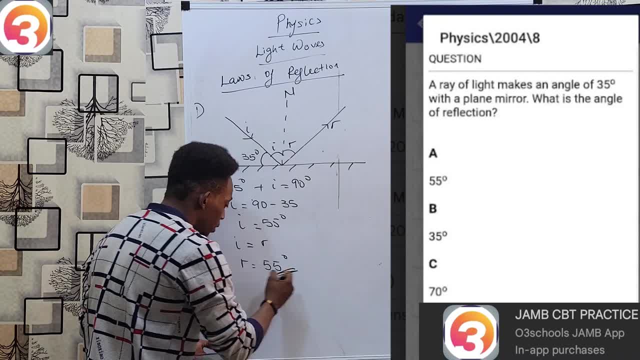 thing was the rect Finite. so, as you have discovered the image of a spot of fact that you beautiful, you can, we can talk at your on the day, both normal and must also be 55 degrees, and that is option A. it is that simple. so, for any, 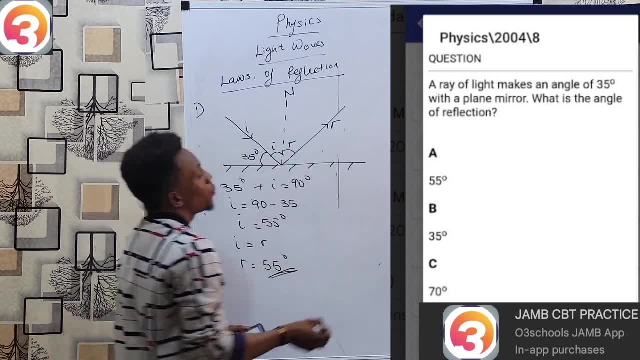 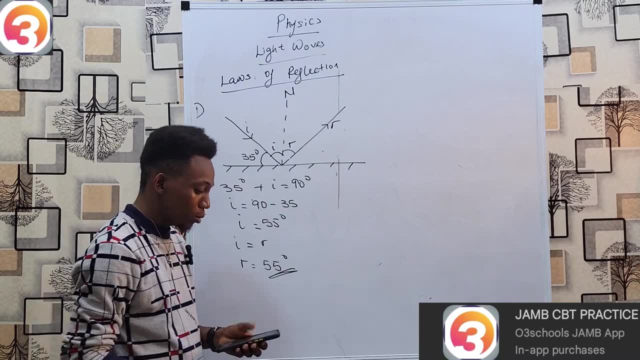 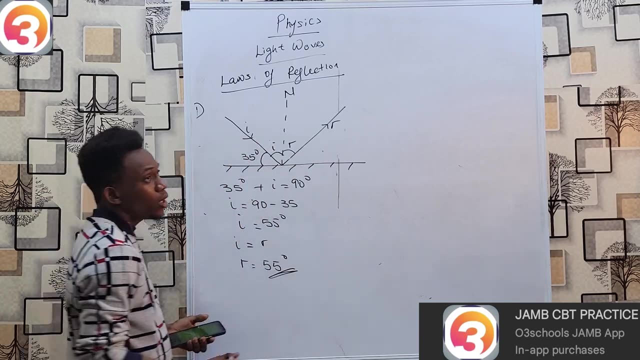 budget being reflected. this is what happens. now. the next social studies. what happens if, during this reflection, I decide to turn my mirror, and by turn I mean exactly rotate my mirror about a certain angle? what happens to the ray? it gets deviated. instead of passing through this expected path, its angle gets shifted. 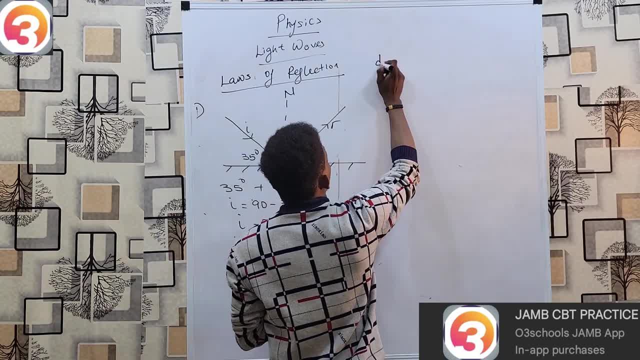 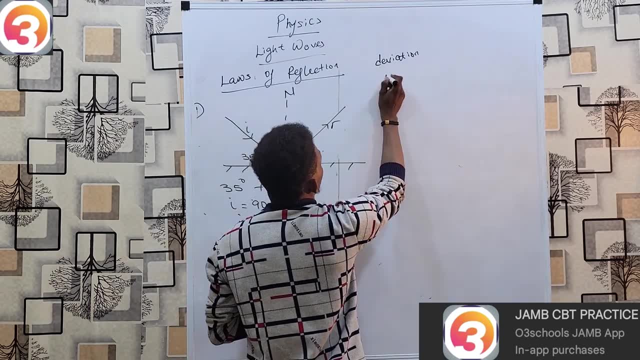 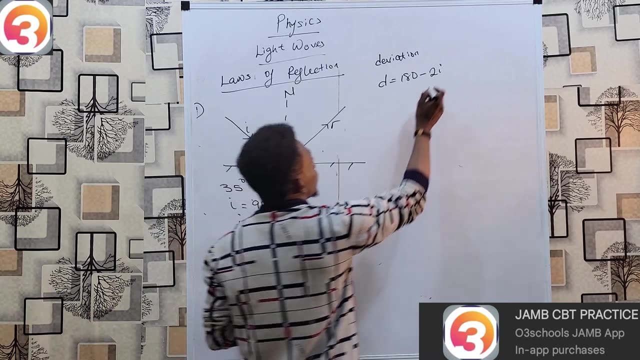 it no longer moves through that and if you are getting deviated, we now have something called the angle of deviation and to get this angle of deviation, the useful formula, which is that deviation equals to 180 minus 2i, 180 minus 2i, and since you know, i equals r. 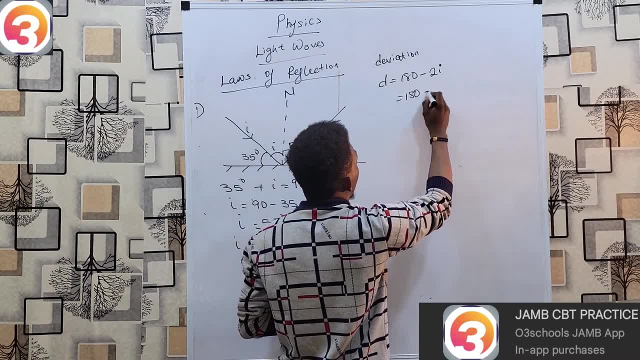 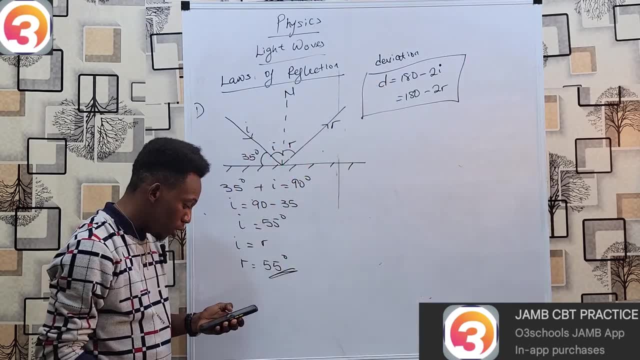 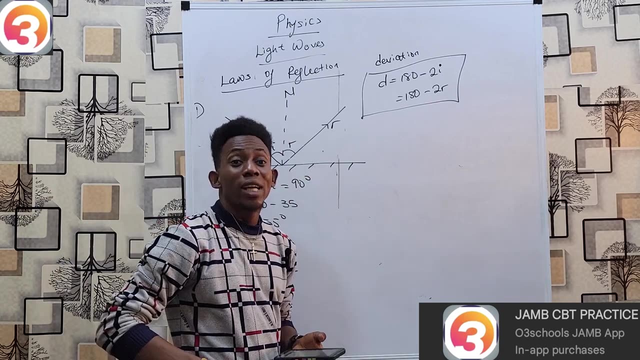 then it shall also be 180 minus 2r, and that gives you the angle of deviation of the ray when the light or when the mirror has been turned, and with that you can apply a question also from this app- and you can see that's why I'm doing this- whereas the 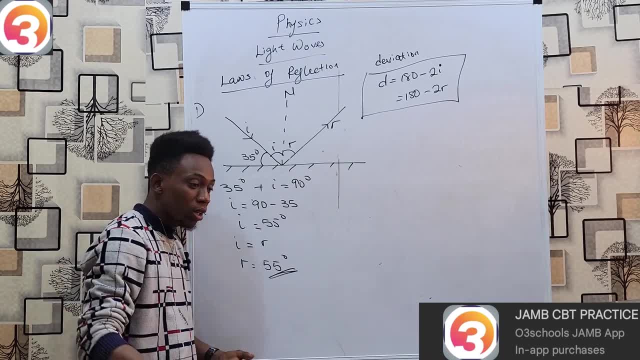 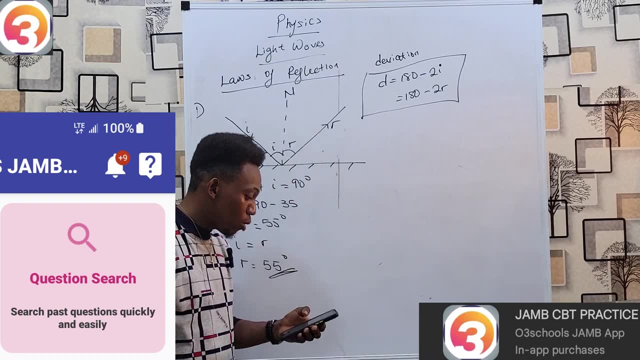 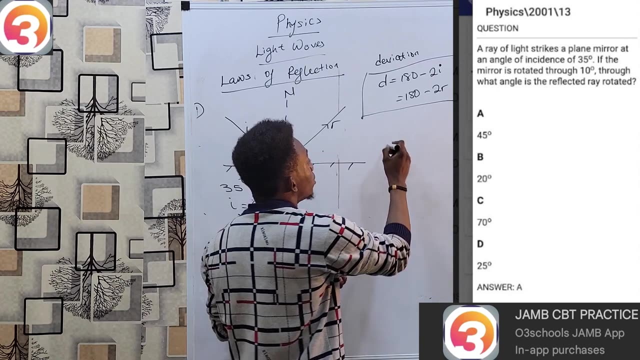 usefulness of the app. as you read, as you learn any topic, you can always come back to this app and search for questions that have to do with that topic you have learned and ensure that your base is totally covered. and now we move on. the question says: a ray of light strikes a thin mirror at an 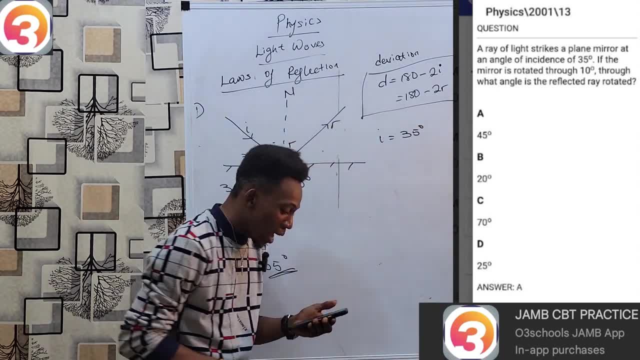 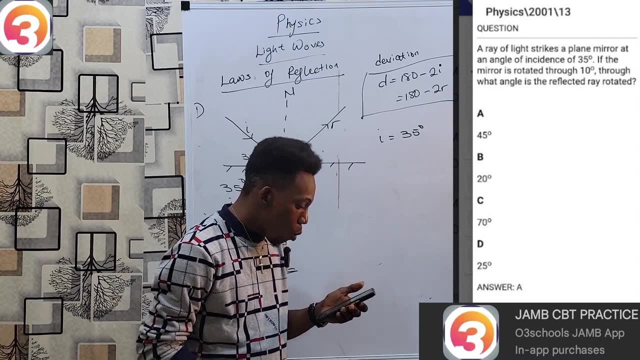 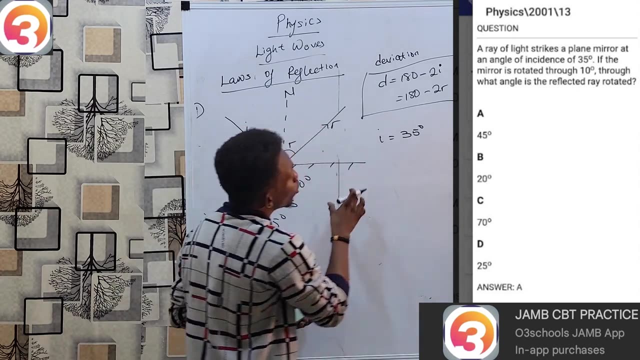 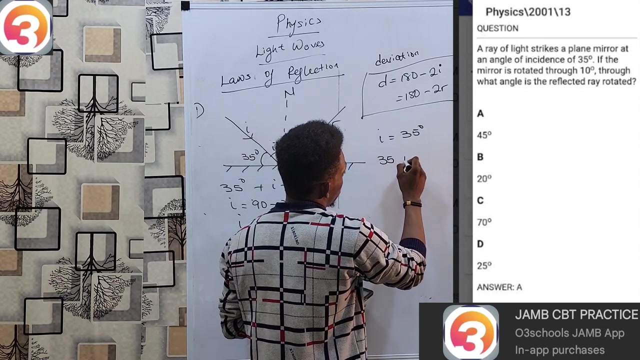 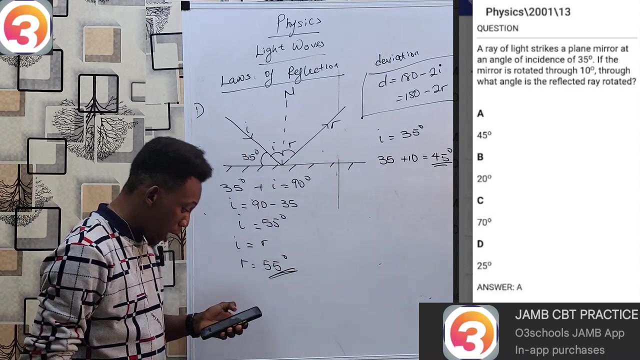 angle of 35 degrees, angle of easiness of 35. if the mirror is rotated through 10 degrees, what angle is the reflected ray rotated? that's what it tells us. that mirror increases its angle by 10 degrees. so our answer would simply be: 35 plus 10 equals to what? 45 degrees, and that's all. and if you look at this notice, 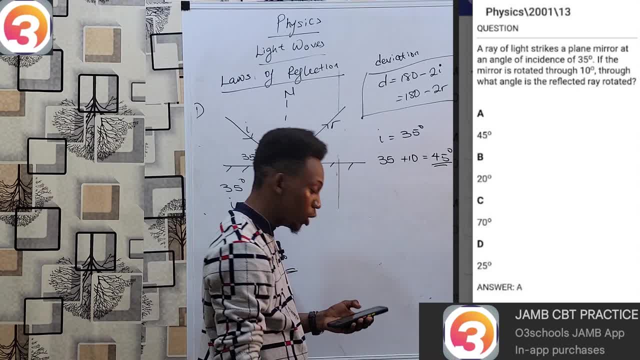 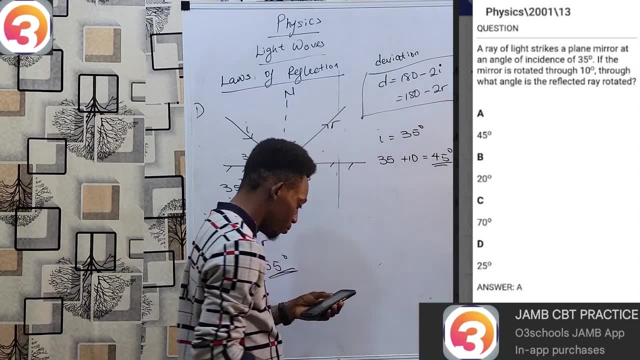 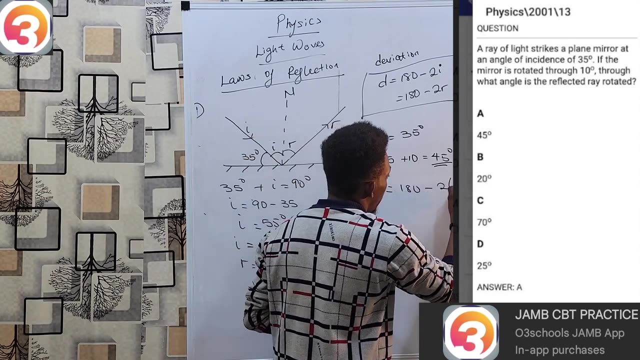 we're not applying this formula because we're not told to find the deviation. if finding the deviation was what we're after, then we would have applied this formula, like you can try it right now. if you have to find the deviation here, the deviation will be 180 minus 2 times. 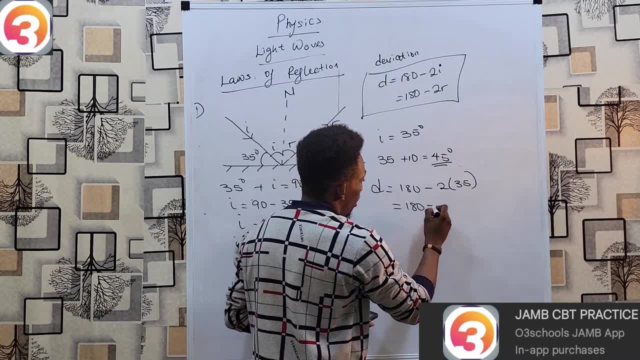 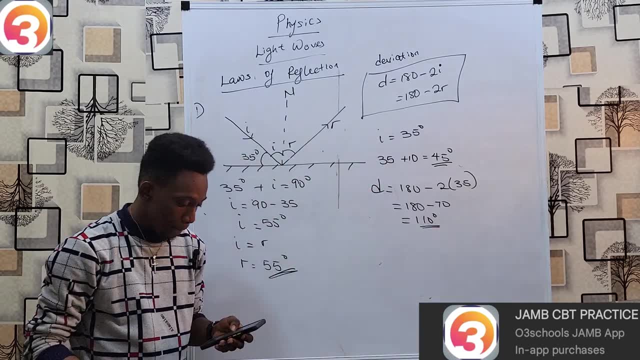 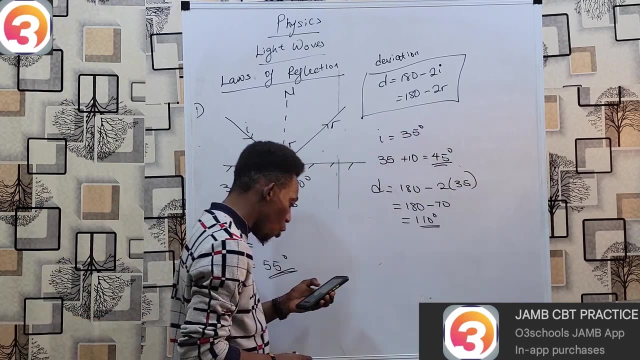 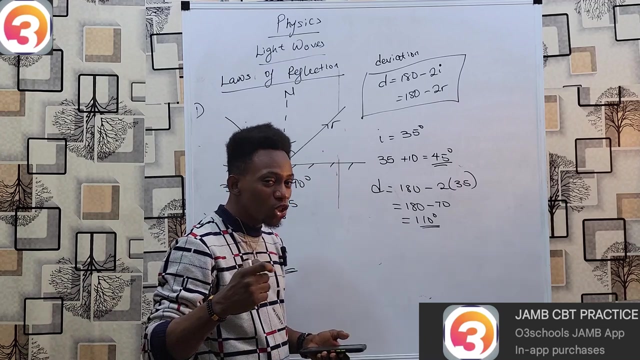 35, which becomes 35. okay, 180 minus 70, which is a hundred and ten degrees. is that okay, all right. so with this we've come to an end of our analysis of plain mirrors. now I have to take one more question just to make sure this is true. Graham Deden, our question now is from 2000, question number: 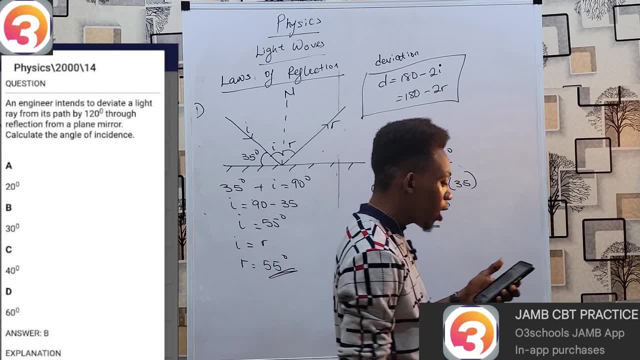 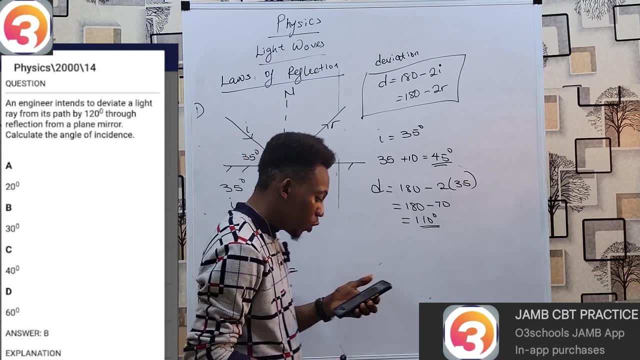 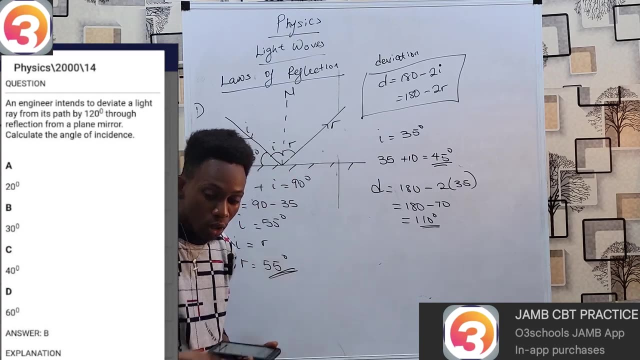 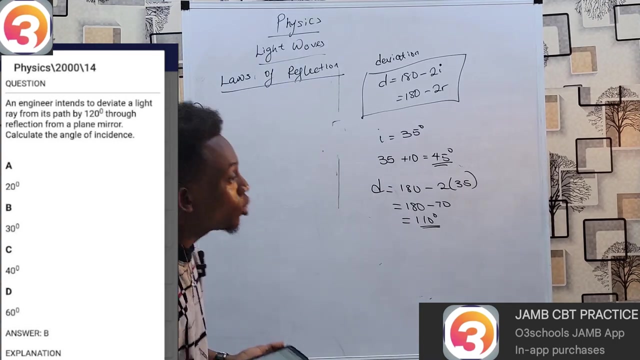 14.. this question is: an engineer intends to deviate a light ray from its path at 820 degrees. calculate the angle of incidence. in this case, we have been told that we intend to create a deviation of 120.. and we want to find the incident rate of incident angle that will be necessary for 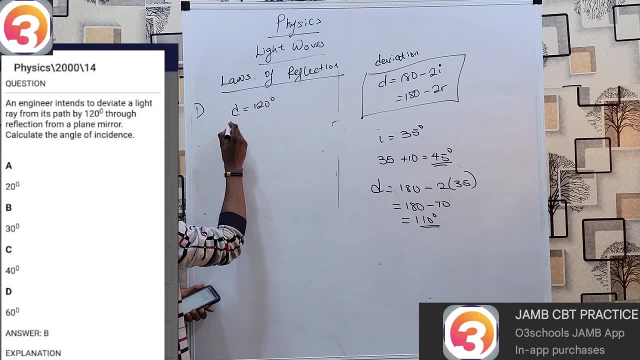 this division. division is 120.. cut c want to find incident angle and to solve that. come and look at this phonological angle of deviation. deviation equals 180 minus 2i. So if my deviation is 120, that will be 180 minus 2i, which I do not know correct like this. 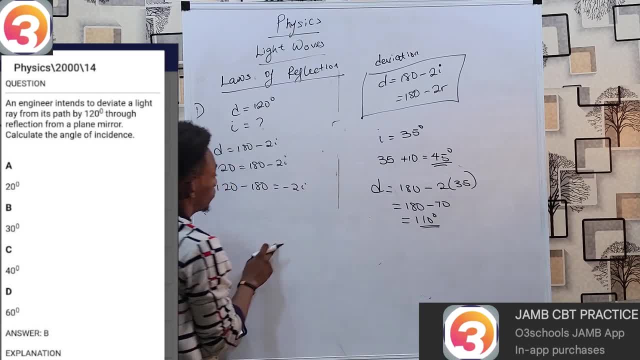 120 minus 180 equals minus 2i. 120 minus 180 is minus 60, equals to minus 2i over minus 2 over minus 2. So our angle of incidence is going to have to be 30 degrees, and that is an answer for option B. and that's what tells you that if